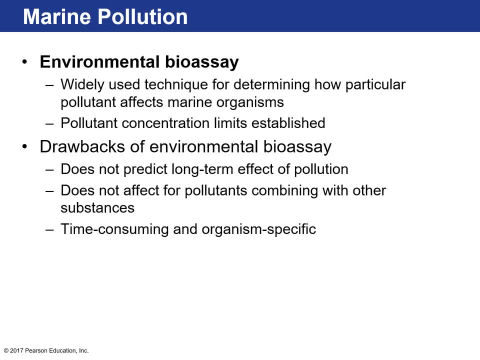 everybody's life and it's going to affect everybody's life and, yeah, it's not good. an environmental biassay is a technique that scientists use, particularly at the epa, to determine how a specific pollutant affects marine organisms, so it can be like a fertilizer. 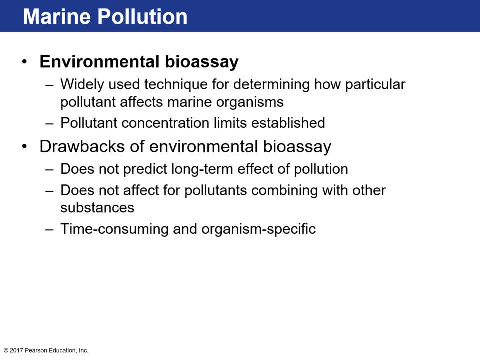 some sort of chemical mercury, for example, or another pollutant, and essentially they conduct experiments with individual organisms and instead they properly mine each of those other pollutants and increase the concentration of %. mortality rate is reached, and that's the pollutant concentration limit that's established. balance, a pretty bad standard given the fact that 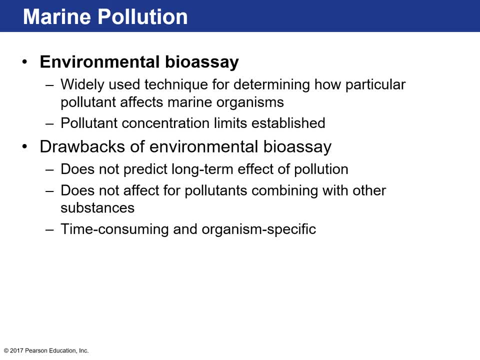 half of the organismsese mortality rate, so half of the organisms have to die at that. idesp lemon deepest for it to b set this standard, the standard, right. so if you're engines to die at that concentration of pollutersish, So if you're just below that standard, so if 48% of the organisms die, then you're like well. 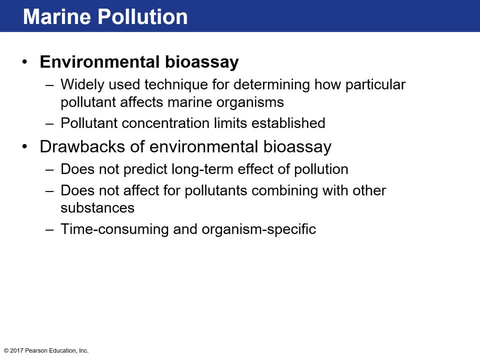 it's below the standard. So there are many drawbacks to this environmental bias, say, One is that it takes into account the kind of instantaneous mortality rate of organisms, So it doesn't look at how it affects organisms in the long term, Because maybe at lower 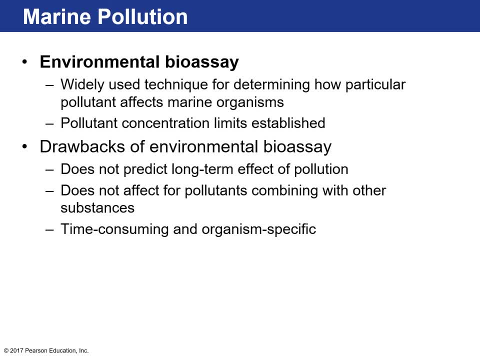 concentrations, the mortality rate is lower. However, maybe this pollutant affects the reproductive rates of the organisms, so that this generation of organisms can no longer reproduce at the same rate as the previous generation. Thus the future generations will decrease in population as a result of exposure to that pollutant. Another thing is that in a laboratory 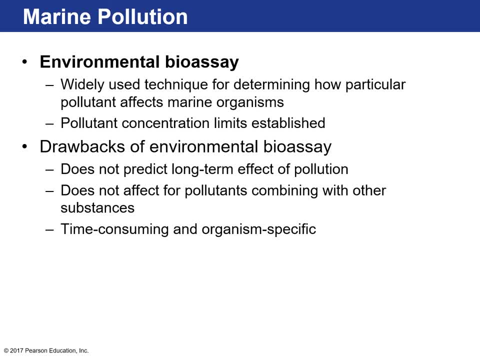 setting. you really just test one pollutant at a time, And so it doesn't take into effect the amount of pollutants that are present in the environment, And so it doesn't take into effect the amount of pollutants that are present in the environment, And so it doesn't take into effect. 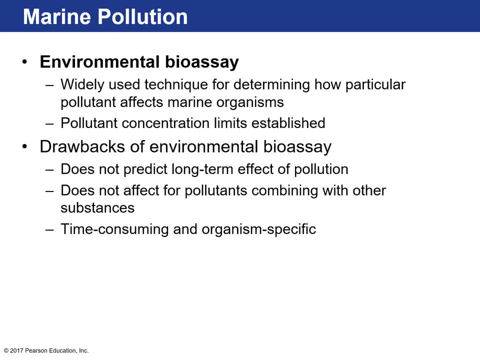 the possible other pollutants that are in the water And that kind of combined effect may alter an organism's biological functions or reproductive functions. And also these experiments are very time consuming, They take a long time to reproduce And they work on one organism at a time. So 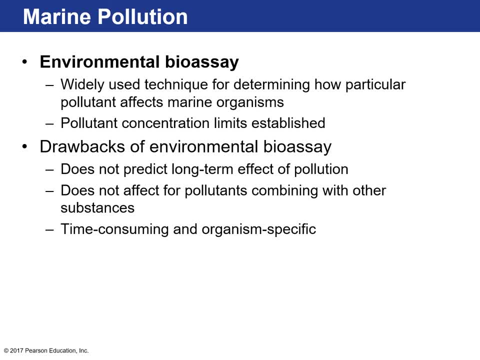 one pollutant, let's say a chemical or fertilizer, may affect sea turtles, But that same pollutant might not affect tuna. So if the experiment was done with tuna, the EPA would set the standard saying that, oh, these high concentrations are okay because it doesn't affect. 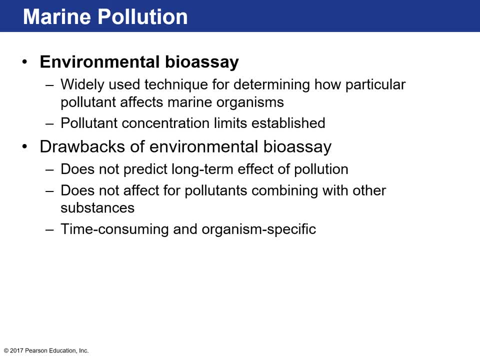 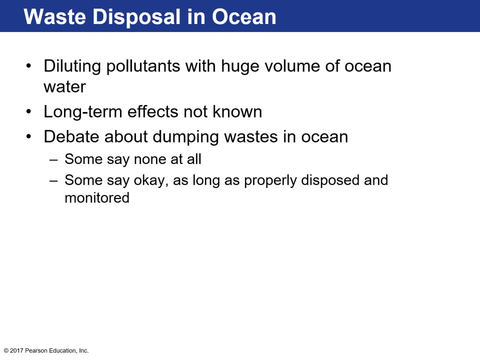 tuna, But in reality it might affect other organisms like sea turtles to a greater extent. So there are a lot of drawbacks to this type of experiments and standard setting. For the longest time there's been a saying: the most effective way to control the environment is to control the 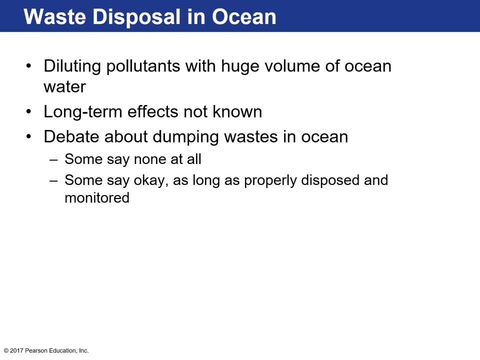 ocean, And that's true amongst people that the solution to pollution is dilution. right, Great rhyming group of words. But really the ocean has always been so vast and so big, So no one's really thought that dumping some trash or pollutants into the ocean would have any effect. But what? 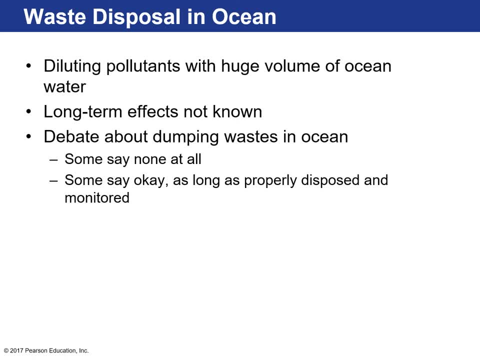 we're realizing now is that, with a growing human population and most people living close to the coastal zones, it's starting to have an effect and we can start to measure how these pollutants are adversely affecting marine organisms and humans. Okay, And there's a lot of debate about 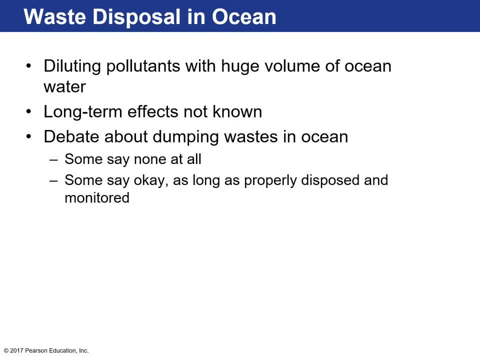 it. I mean it depends on the pollutant. Not every pollutant is the same, but some oceanographers- actually a lot of oceanographers- say that we shouldn't be polluting the oceans with sewage and all kinds of trash, Or not at all. Other 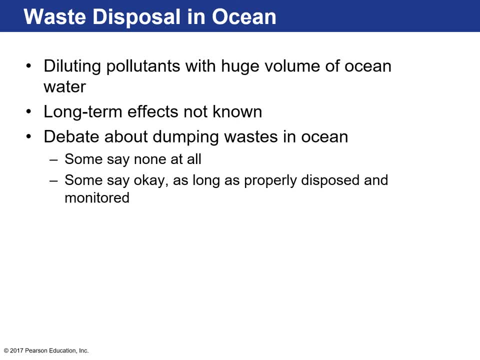 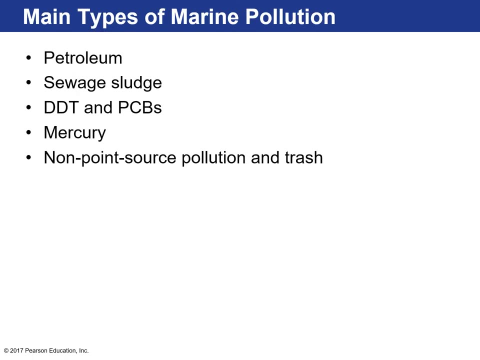 say some is okay depending on the pollutant. but you know that's still debated. But everyone agrees that if we're sending out material into the oceans or pollutants, it has to be monitored. Okay, So here are the main types of marine pollution. There's petroleum or oil, Okay. 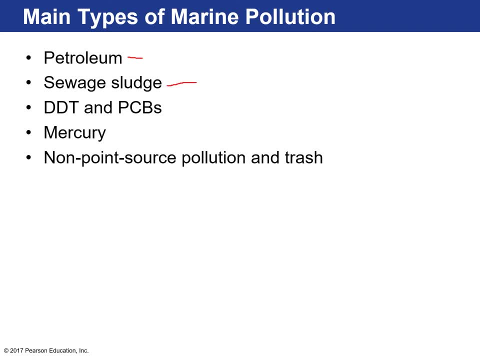 There's sewage sludge- Okay, This is the material that's our number one and number two. bathroom material: Okay, This sewage water typically goes to treatment plants. It's chlorinated and filtered and all the heavy material sinks out of the water, And then that's sewage sludge. It's just the. 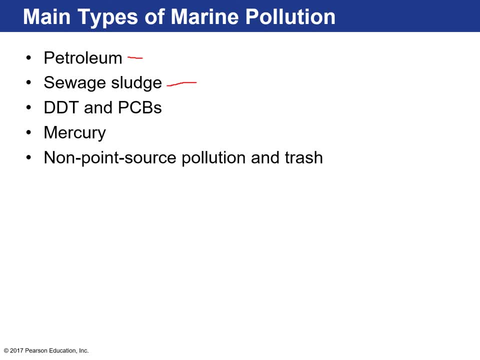 solid matter from our waste, Okay. Then there are: DDT is an insecticide, Okay, So that's chemical- And PCBs- These are industrial chemicals that we use to create or we used to use to create refrigerants And we used 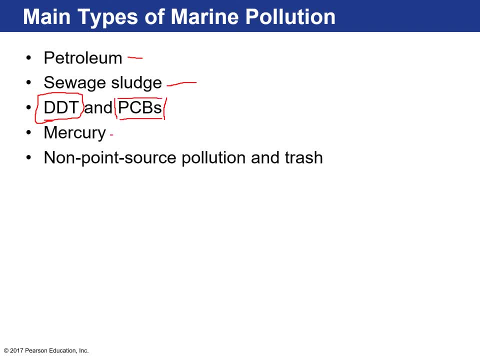 in transformers? Okay, Mercury is a very common element. It's a metal that's kind of liquid in standard pressures and temperatures, But it's used a lot in different industrial uses, and also as a byproduct of burning coal. Okay, And then non point source pollution. 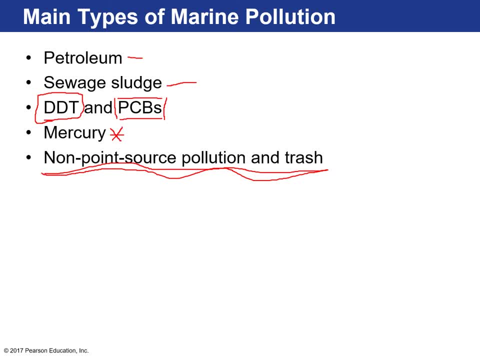 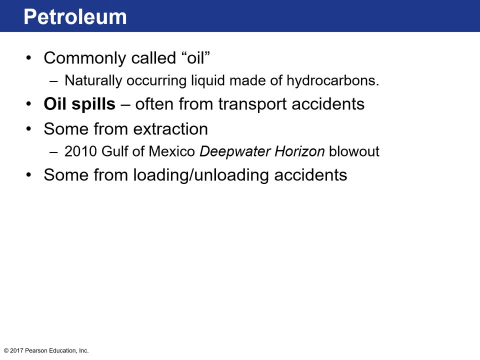 And trash. This is material that can't be traced back directly to a source. Most of the time it's plastics. All right, Let's talk about petroleum first. We call it oil. It's actually naturally occurring. Okay, It's a liquid made of hydrocarbons, a lot of carbon. 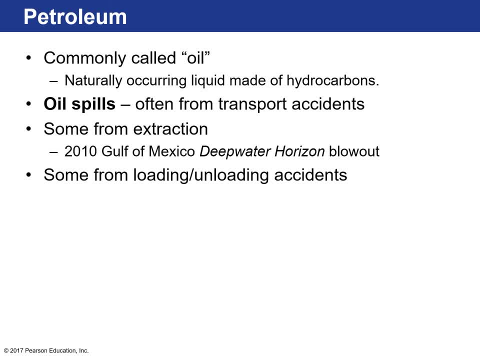 lighter hydrogen in it. Essentially, it's the lots of organic matter, typically from marine organisms, that, like algae, that live on the surface of the ocean- Diatoms, for example, on the surface of the ocean floor- And, if enough of them, accumulate over time and are buried by. 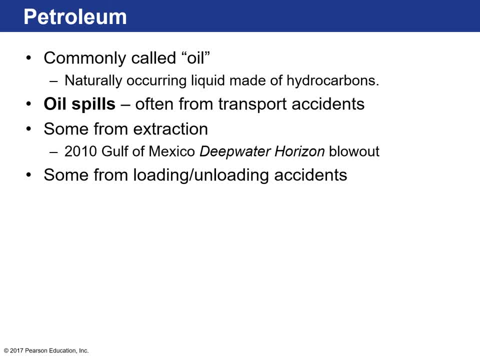 sediment, the organic material, can become hydrocarbons. Okay. So in terms of marine pollution, it becomes a pollutant when it spills into the ocean, and in vast quantities. Most of the time it's transportation accidents. Sometimes the accidents can happen from extraction, because we go. 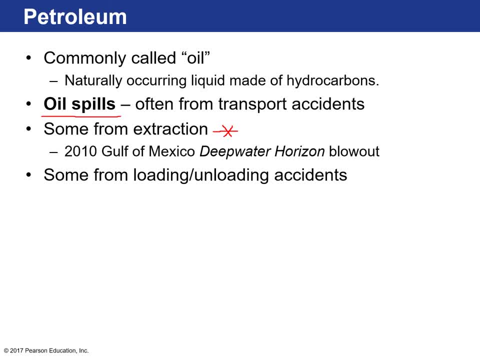 out to the ocean- Kind of offshore platforms and drill wells- And sometimes there can be accidents like explosions. The craziest and greatest example of this was the 2010 Gulf of Mexico Deepwater Horizon blowout. There's actually a major motion picture on this event And Mark Wahlberg is the 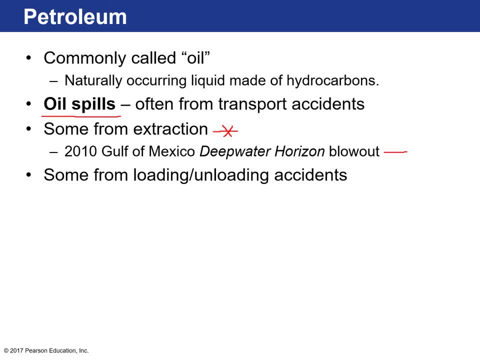 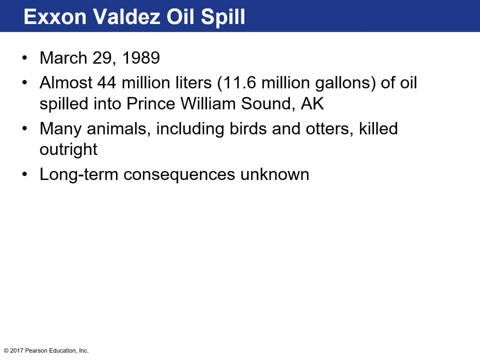 protagonist in that movie, Marky Mark Right, And other. smaller spills occur when large boats that transport the oil spill, some during loading and unloading. Okay, The first you know major oil spill that occurred and kind of encompassed the consciousness of you know. 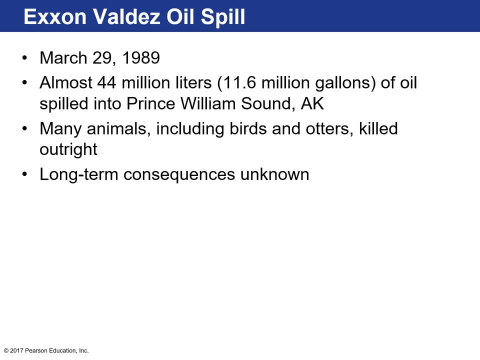 the human sensationalism on the media and stuff like that was the Exxon Valdez oil spill And that was in 1989. About 11 million gallons of oil spilled into the beautiful pristine waters of Prince William Sound, Alaska, okay, and this area is absolutely. 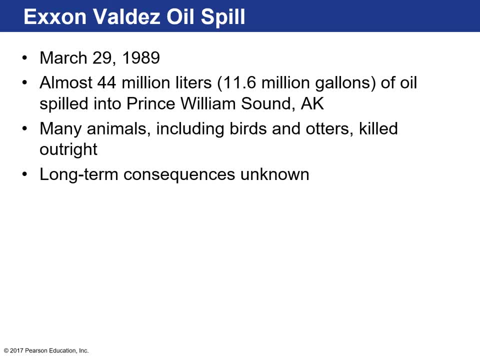 beautiful, you know, very untouched, very natural, and this thick crude oil just spilled everywhere. what happened was one of the boats that was leaving Valdez was trying to avoid some icebergs and they veered off course and they struck some rocks that were kind of jutting out from the seafloor, and so all of this crude. 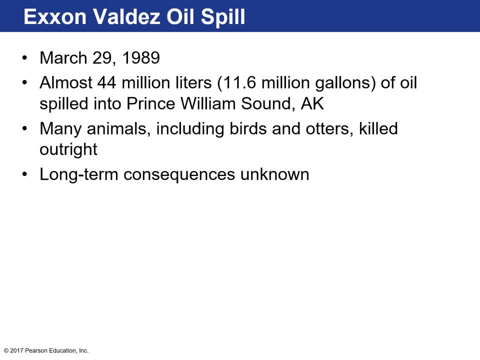 oil just spilled along about 11 kilometers of coastline in Alaska, just caked it in oil. so many of the animals- birds, otters- were almost immediately killed as they were covered with oil. okay, so the immediate impacts of oil spills are pretty drastic. and if you see the pictures, if you see the 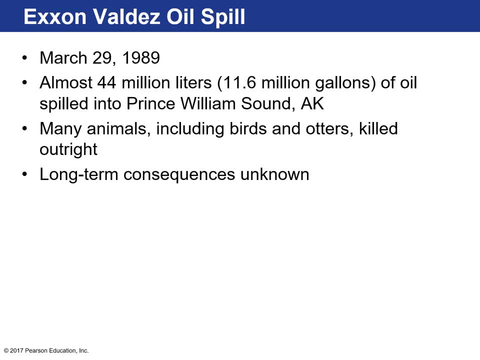 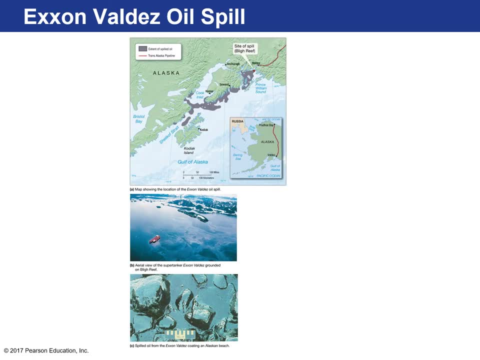 you, you media coverage. it's sad, okay. so the immediate impacts are quick and and devastating. the long-term consequences are kind of unknown. here's that 11 kilometer part of Alaska. it's essentially right on the border with Canada. this entire area was covered by an oil slick. okay, here's another image. 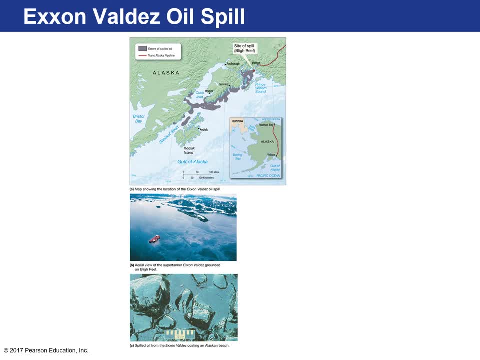 you can see here. here's a close-up image of the emulsified oil that spilled, as this tanker just ruptured and spilled its guts all over the coastal waters of the Gulf of Mexico and the Gulf of Mexico and the Gulf of Mexico and the Gulf of Mexico. 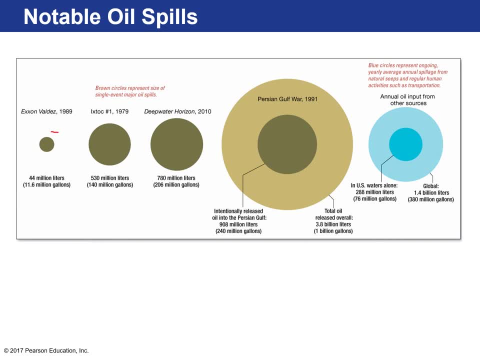 okay, so here's the Exxon Valdez spill in terms of volume of oil that was leaked into the ocean in in one moment. okay, so you know, 11 million gallons. there have been other kind of single event, major oil spills that have been much larger. okay, ten years before this, in the Gulf of Campeche, in the Gulf of Mexico, I'll. 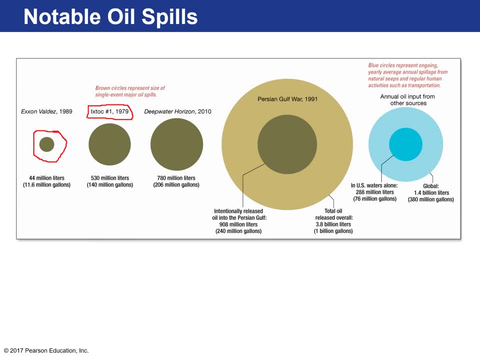 go off the coast of the Yucatan. each took the Mexican petrol arrows, had a blowout in one of their wells and about 140 million gallons spilled in the Gulf of Mexico. okay, and some of that stuff even made it to Texas at that time, okay. 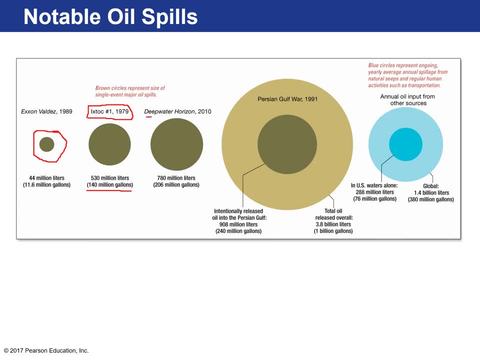 the Deepwater Horizon blowout, which was that major motion picture. this spilled about a two hundred and six million gallons into the Gulf of Mexico. this was pretty crazy. crazy because this spill was really large, unintentional obviously, the there was just a huge blot and the platform kind of collapsed, but every four days it 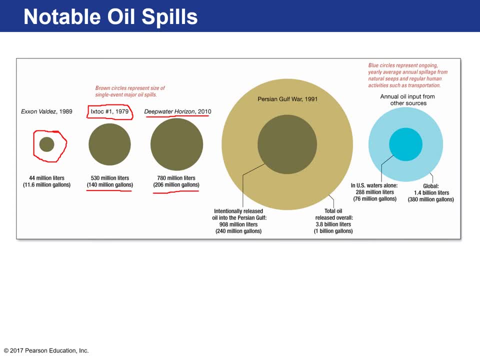 released an equivalent of the Exxon Valdez spill into the Gulf of Mexico and that really dirtied a lot of the Gulf Coast beaches in the panhandle, Florida, Louisiana, Alabama, Texas, I mean you name it. those, the people who live and work there were really affected by this. 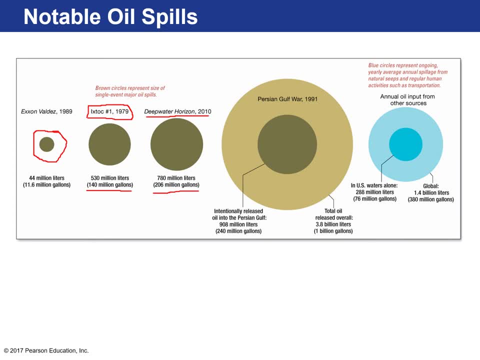 And what was crazy too, is, at that time, they actually had a camera where the blowout occurred- underwater, and so, in 2010,, you could go and go to the live stream of this oil just spilling into the Gulf of Mexico, which was pretty crazy, and ended up capping that blowout. that blowed up, well, using submersibles and robotics to do that, which was pretty crazy. 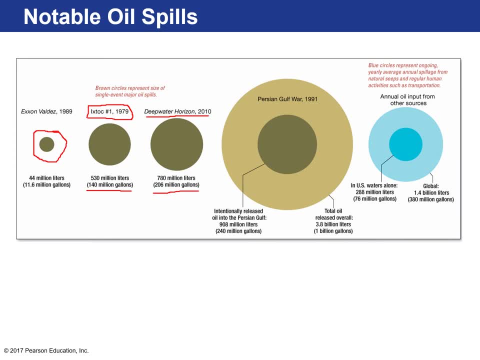 Okay, another. this was an intentional release of oil into the ocean as a result of the Persian Gulf War. What happened here is: Iraq invaded Kuwait- Kuwait's, this tiny little country that you know the spare of the history lesson- was part of Iraq at one point, but then US intervention, it became its own country, really close to the Persian Gulf, very tiny, very oil-rich. 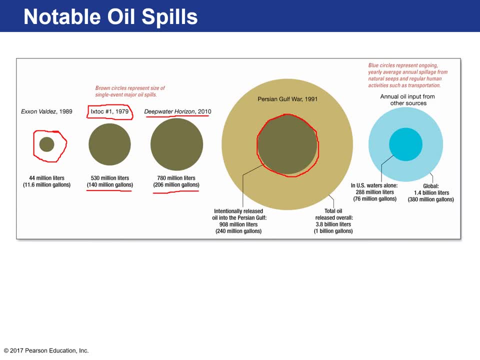 Okay. so Saddam Hussein came in. He came in and kind of invaded Kuwait and that's what started the Persian Gulf War. and so when the US went to Kuwait and kind of kick out the Iraqi soldiers like a scorned lover, they essentially just lit the wells on fire. 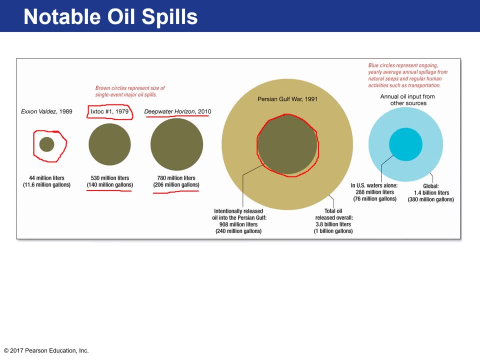 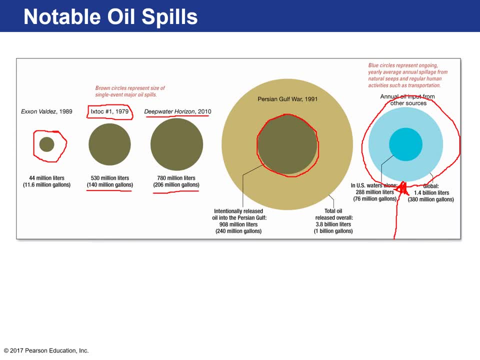 That happens, naturally. But the difference is is these are you know these spills occurred in one small area, you know, in the ocean. So it had a dramatic effect on the local organisms. But this is just you know, drops being emitted in many different parts of the world's oceans. 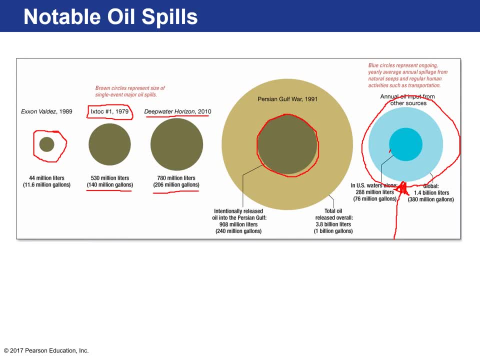 So in an entire year, natural seepage accounts for about how much oil was released from the deepwater horizon. But again, this occurs naturally, And when it occurs like this, it's just really small amounts in different parts of the ocean all over the place. 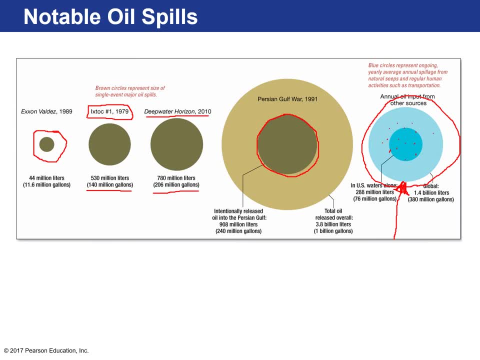 And that allows the bacteria to kind of break it down so that it doesn't affect marine organisms as much. Okay, US waters alone is a lot. We have a huge continental shelf that has got a lot of oil in it. Okay, 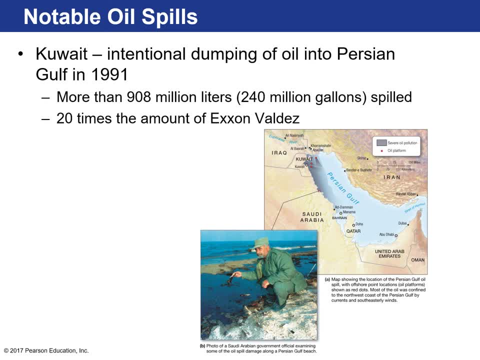 So here's Kuwait. This was in 1991.. So there was a lot. Here's the entire kind of extent of that oil slick that was released into the Persian Gulf, which was a shame. Some of these areas have beautiful coral reefs. 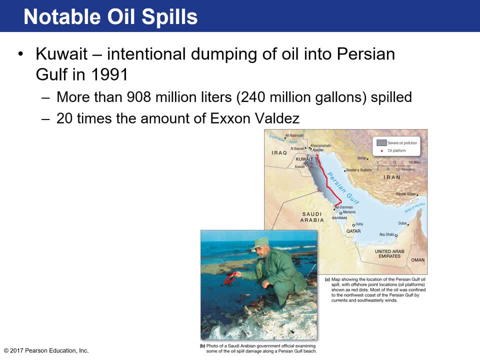 You can see this guy's dipping his fingers covered in crude oil, But yeah, about 240 million gallons was spilled into the Persian Gulf as well, as there were fires that lit up and blackened the sky, which is pretty crazy, Okay. 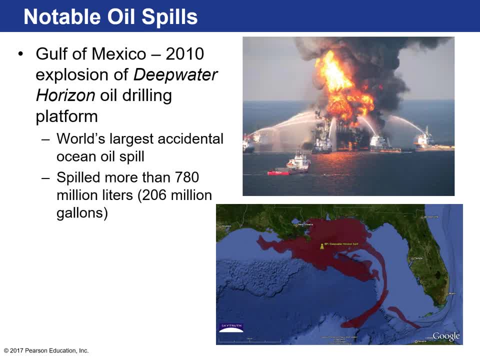 And that was 20 times the amount of exon. Well, that's okay. Here's the deep water horizon. This is where Marky Mark, you know- courageously jumped into the water after the explosion. Okay, But this was one of the platforms off the coast of Louisiana, right here. 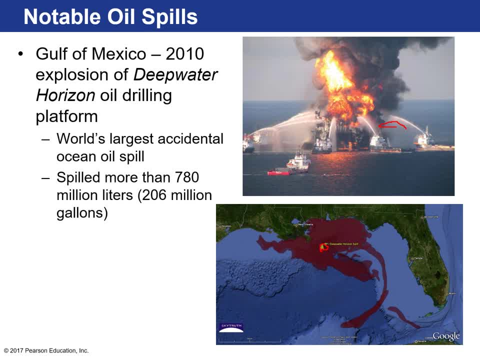 And there was an explosion And afterwards they realized that was mostly due to negligence. BP is taking responsibility for it, And this oil slick covered a lot of the Gulf Coast communities here, Killed the fishing industry in a lot of these places. Florida is dependent on a lot of tourism. 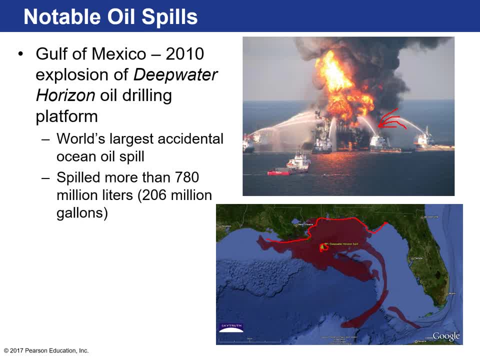 And oil was just washing up ashore in these areas. So that spilled about 206 million gallons of oil, And that's in our own waters here in the US. Okay, Then here's the Ishtuk one. This occurred right here. 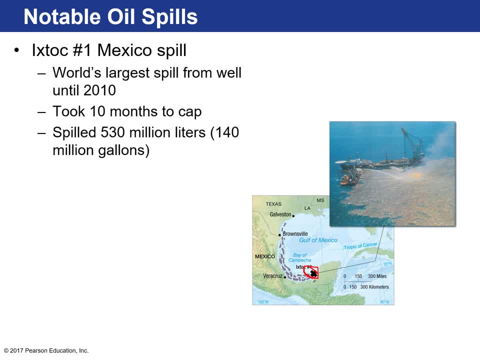 See, Really close to the Yucatan And this oil slick kind of traveled all the way to Spring break spots like South Padre Island, Brownsville, Texas. It's pretty crazy: 530 million liters. This didn't receive as much media coverage like the Exxon Valdez spill. 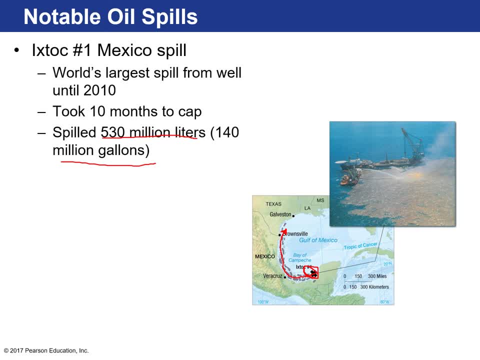 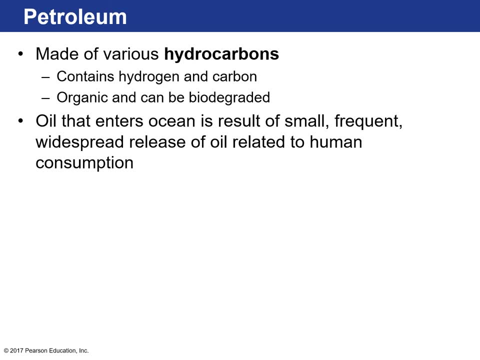 But still a very notable, large, unintentional oil spill. Okay So petroleum, really, it's made up of a lot of hydrocarbons And that's a natural substance that occurs in the oceans, On continental shelves, naturally. Okay, So it's organic. 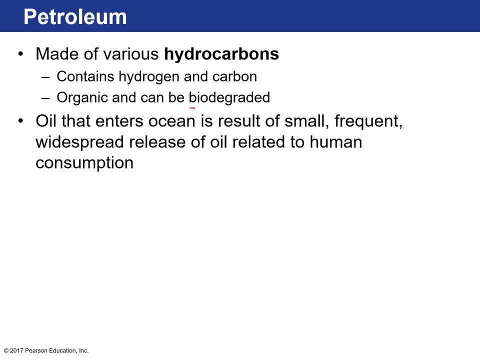 And what that means is that it can be biodegraded, meaning that, you know, small bacteria actually can break it down. So when oil enters into the ocean, it's a natural process and the microbes get into it and break it down. 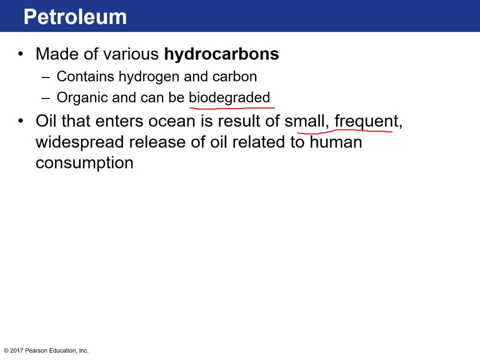 So when it occurs in small, frequent kind of releases, like natural seeps, this is completely normal, Okay. However, When it When it enters into the ocean via those major oil spills, the effects on marine organisms is drastic in the short term. 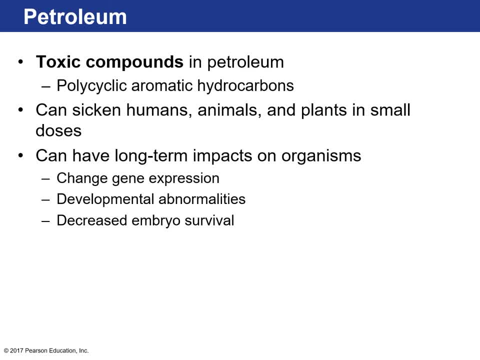 Okay Long term. we don't really know that much, but it's because petroleum is a toxic compound. It contains a lot of different chemicals in it. It's like a big mix of different chemicals. One of the worst ones is PAHs- polycyclic aromatic hydrocarbons. 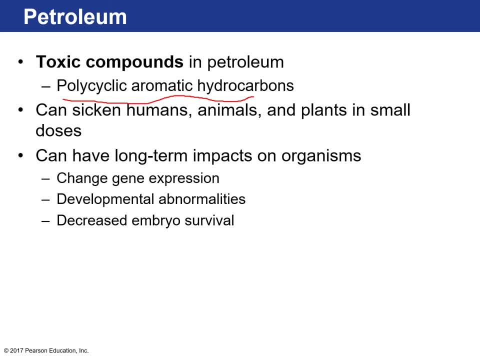 And this has been shown- to change the gene expression in organisms, So cause mutations. That's not good. Also, lower fertility rates. That's not good. It's sickens humans and animals Okay, And they can have long term impacts on organisms. 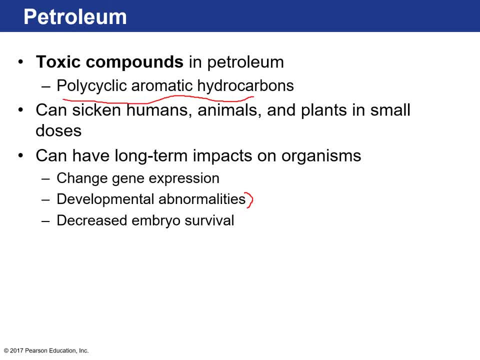 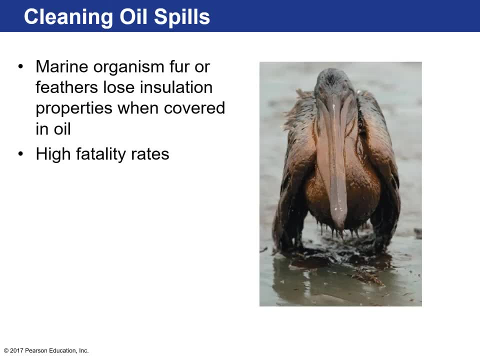 They can develop abnormalities. if you're exposed to PAHs for too long and decrease embryo survival, That's not good, All right. And then I'm sure you can Google the Exxon Valdez spill. There are a lot of pictures from that time showing a lot of the marine birds that were. 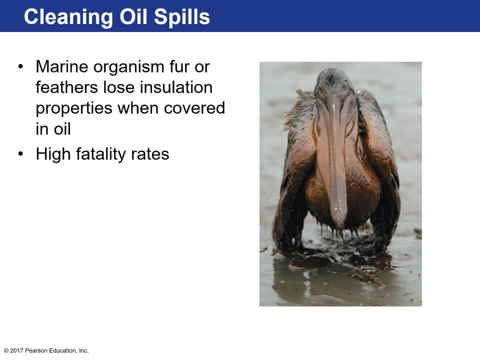 infected by the crude oil. Here this is a pelican just covered in the oil- Really devastating. What happens is, when they're covered by that oil, their feathers are no longer, as they don't insulate their bodies as well. So overnight these birds basically just froze and cooled down to death because they were. 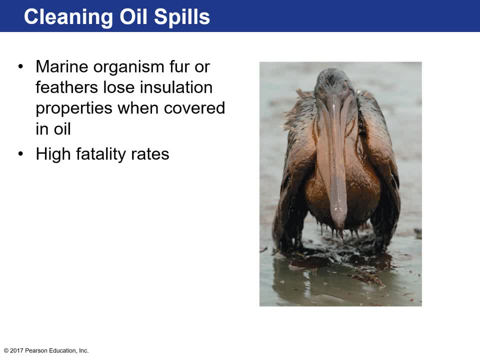 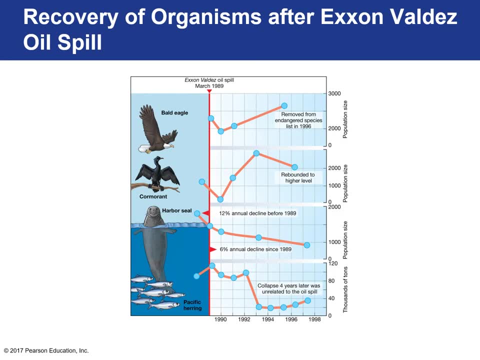 just covered in. that oil, Okay, Caused really high fatality rates in marine birds. Okay, But it's a short term, Okay. So here are three different organisms that exist off the coast of Alaska And as a result of that oil spill, which was devastating populations of the bald eagle. 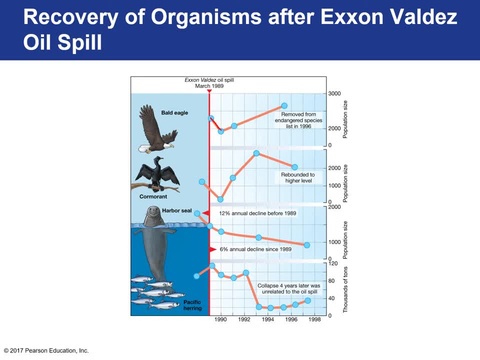 decreased rapidly from 89 to 1990.. So did the, so did cormorants, and harbor seals, And the Pacific herring actually saw an increase in population, But this is the immediate effect. This is within one year, Okay. 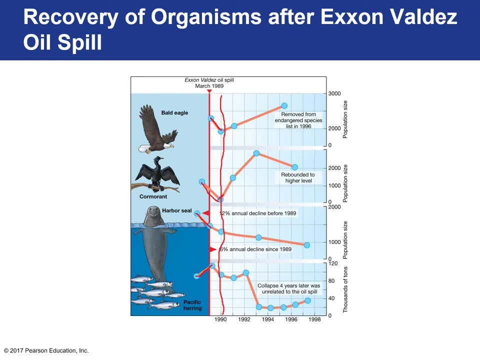 And then after one year the populations actually rebounded fairly quickly. Okay, Bald eagles increased drastically, And so did the Pacific herring. Okay, The kind of collapse of the Pacific herring in 1993 was associated with the disease. 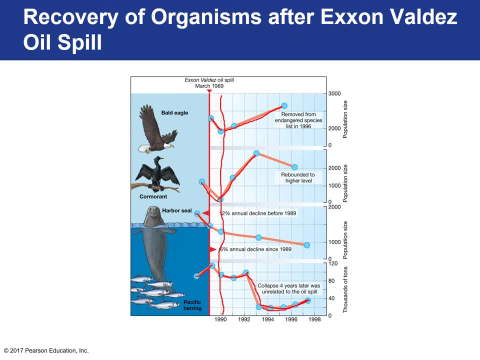 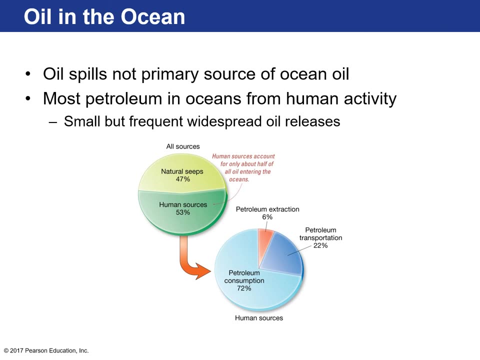 So it was unrelated to the oil spill. but you know, after the oil spills there's kind of an immediate effect on marine birds, So they typically bounce back fairly quickly after a few years. Okay, Oil spills- even though those are kind of drastic one time- events that occur in the 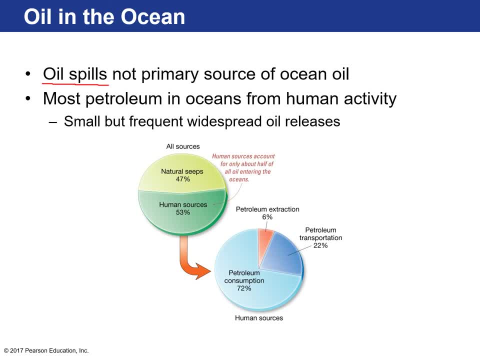 ocean and are devastating to that local area. If you add up all the oil being spilled into the ocean, that's not the primary source of all the oil. Okay, When you look at human sources in the ocean, which makes up more than half of all the oil? 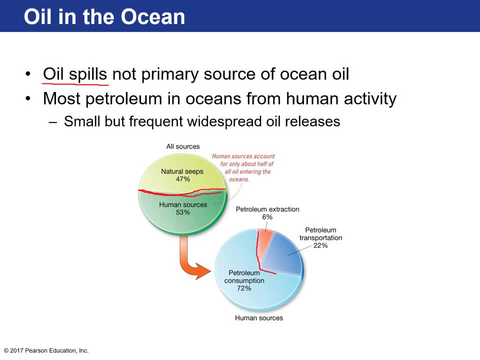 in the ocean. Okay, Petroleum consumption: This is us guys driving our cars, boats, cruise ships, spilling, you know, oil onto the street and that runs off into the ocean. That's most of it. Extraction: the wells blowing out and spilling that occurs. that's only about 6%. 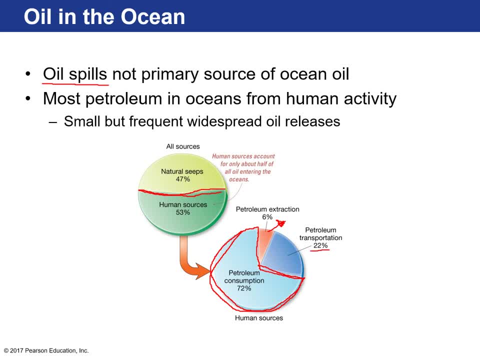 And then this is transportation- about 22%. So that's the oil tankers and the spilling that occurs there. Okay, So most of the petroleum in the oceans is because of us. We're guilty, But and it's- and it's really small but very frequent oil releases that it contributes. 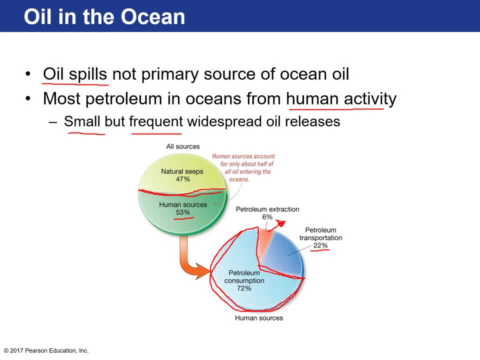 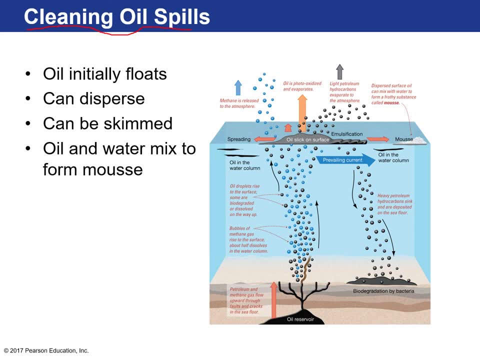 to us right here: 53%. Okay, Now the cleaning of oil spills. we've learned a lot since the Exxon Valdez spill. When that happened, what they did- and same with the Deepwater Horizon spill in 2010,- what a lot of the oil companies paid for was to go out and dump oil. 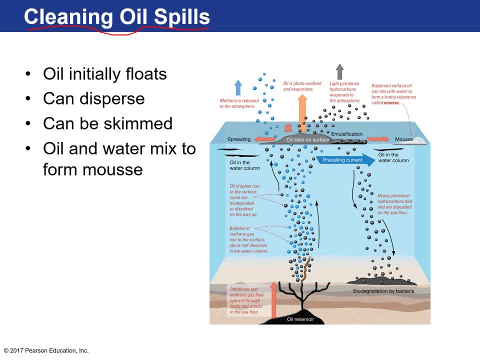 Okay, And that's what they did. And the same with the Deepwater Horizon spill in 2010.. They went out and dumped chemicals on top of the oil slick. Okay, So here's the oil slick. They would dump dispersants. 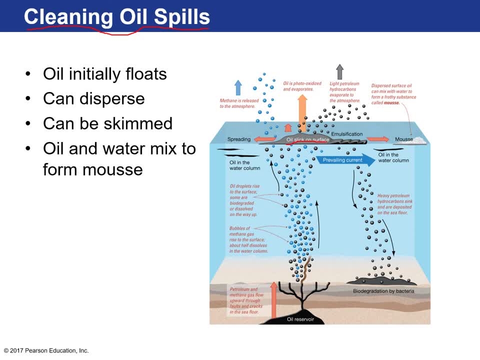 And what dispersants do is just spread the oil out. so it doesn't like thicken up Now, so that doesn't really like clean it up, That just kind of dilutes it and spreads it out. So what they found was that wasn't really particularly effective. 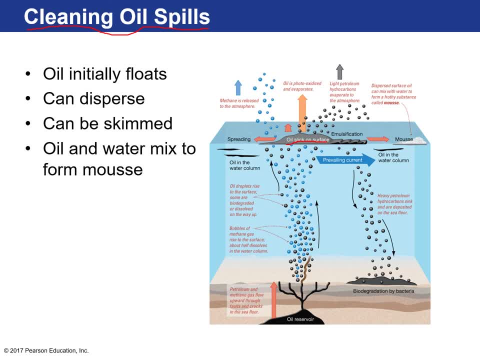 In Alaska during the Exxon Valdez spill, some of the people on the ground went out and started essentially like using pressure washers- really hot water- to kind of disperse the oil right on the coastline And that looked great, but it actually killed a lot of the marine organisms, like the mollusks. 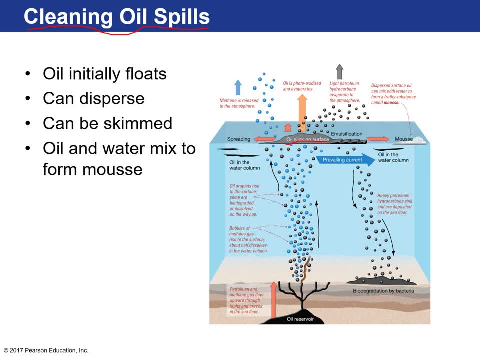 and the barnacles that existed on the rocks And areas that weren't treated in that fashion- with dispersants or really hot water- actually recovered slower than areas that were just completely left alone. Okay, So what happens is oil, because it's a natural substance. microbes will get to it and break. 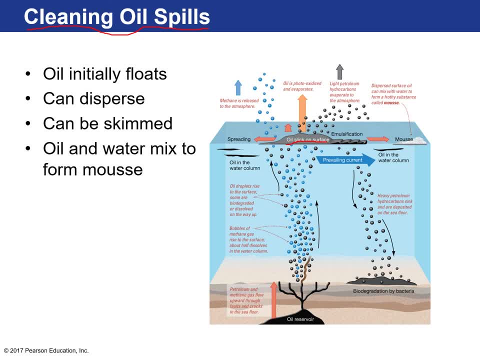 it down and clean it up eventually. So weirdly or oddly enough, leaving the oil alone is actually a better process than actually trying to actively clean it up. I mean, obviously like, what happens with oil is when you initially spill it, it floats. 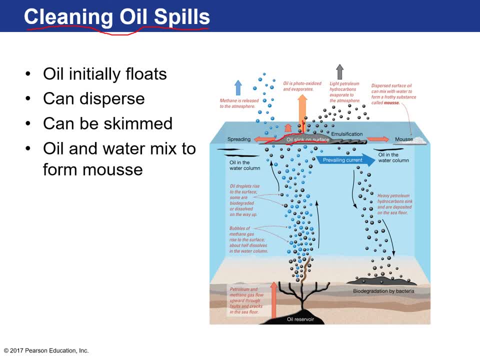 because its density is less than that of water. Okay, Then a lot of the volatiles evaporate away. Okay, Then it oxidizes and it goes into the atmosphere. And so what happens? there is, it begins to emulsify. Okay. 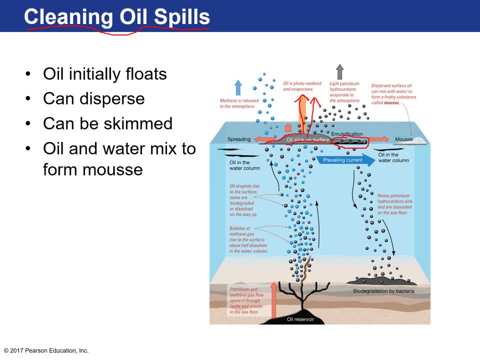 And it thickens into this thick kind of oily substance. This can be cleaned up, It can be skimmed out, and that's a good way of cleaning it up. Otherwise it gets too heavy and then starts to sink and goes right back and deposits on. 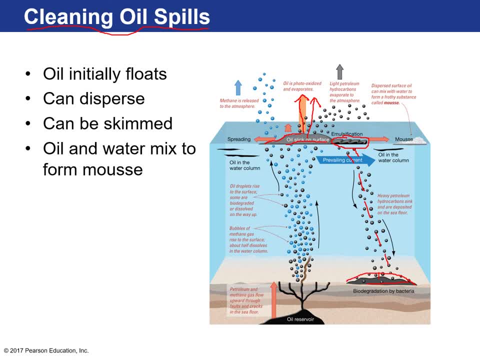 the ocean floor where it'll be degraded or biodegraded by microbes. Okay, When it mixes around a lot because of ocean currents and wind, it turns into this kind of thick mousse, which is pretty gross, Okay, But essentially it spreads around. 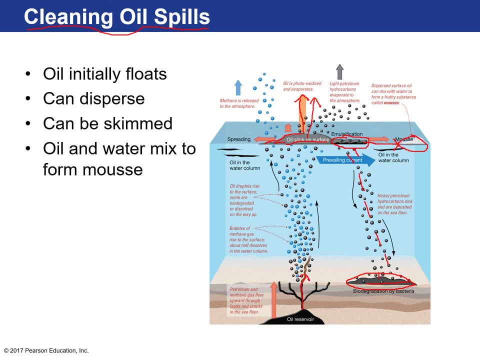 This is an oil reservoir in a natural seep, Okay, And so this is how it's really slowly into the ocean and allows for biodegradation to occur, Okay, So, yeah, we can skim it, But ultimately, biomediation is the best method in cleaning up oil spills like this. 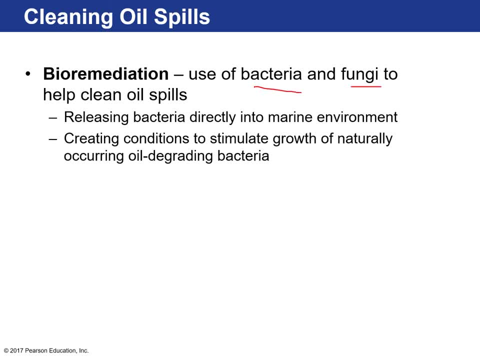 Okay, The use of bacteria or fungus to clean up those oil spills. So what we can do is actively release bacteria into these areas and help them concentrate around the oil spills to break it down faster, And that's proven to work really well. Another method is like introducing fertilizers that are favorable for bacterial growth into 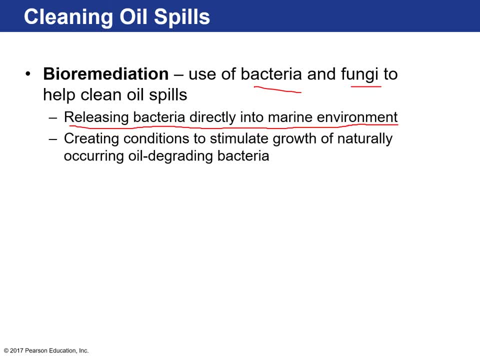 these areas And that has shown to accelerate the breakdown. Okay, Okay, So that's a lot of oil, naturally, and that really stimulates the growth of that degrading bacteria. All right, So that what we've- The research that's been poured into this area- has really found that bioremediation. 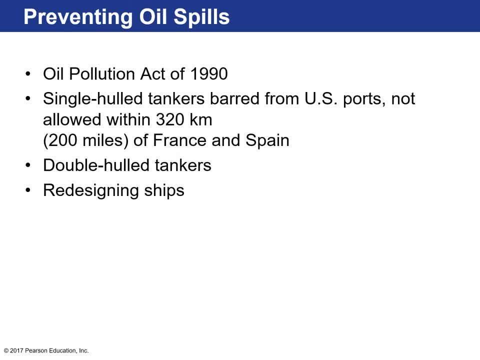 is really the best way to do it. Okay, So since the Exxon Valdez spill in 1989, there were a number of legislative acts that were passed that were very important. All the new tankers had to be double-hulled instead of single-hulled. 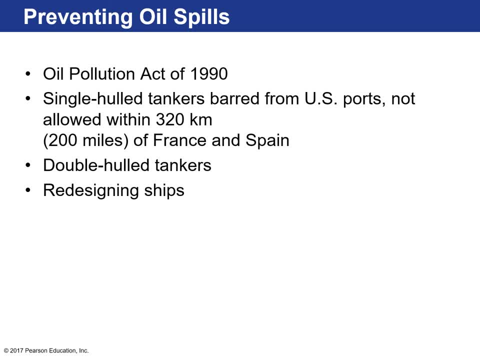 Okay. What that essentially means is there's a second layer of protection. So if a boat ever runs aground again, it might pierce the first hole but it might not get to the second hole where the oil is stored. And in addition to that, now the oil tankers have to have multiple compartments. 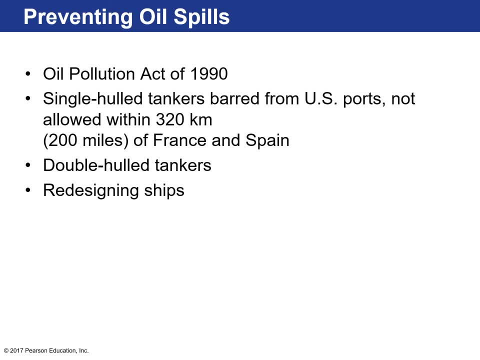 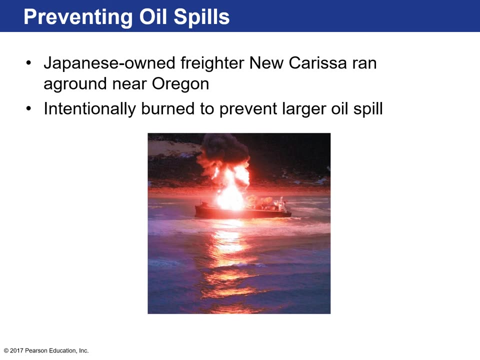 So even if it runs aground and the second hole is pierced, only a portion of the oil would spill into the ocean rather than the entire tanker. Okay, So it's really redesigning ships, Okay? One really crazy example of an oil spill was a Japanese tanker that was off the coast. 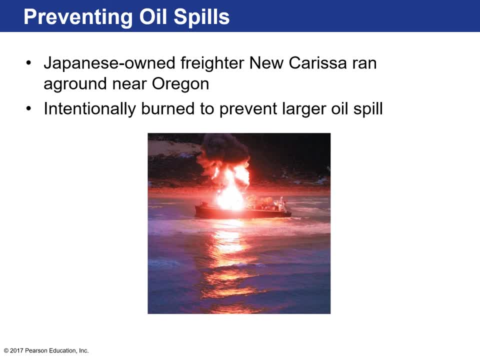 of Oregon. And what happened here was it kind of ran aground and it was kind of being pushed by the ocean onto land and was starting to spill oil. So what they decided to do was to light it a fire, To just burn the oil. 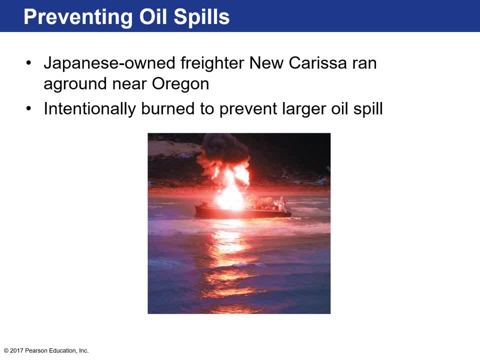 Okay, All right, So they decided to let that stuff spill off and let that stuff go into the atmosphere, rather than let it spill on the coastline of Oregon. Okay, Eventually that fire kind of split the Japanese tanker in half and there was a spill. but 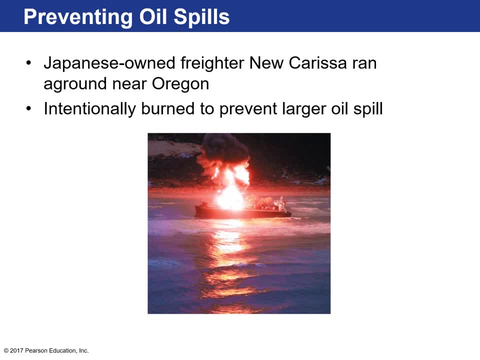 they estimated that they prevented about half of the oil from spilling onto the Oregon coast. And then, what was pretty crazy, then they towed the boat out to deeper waters and then they sank it with a torpedo, which is pretty cool. So that was an intentional burn to prevent, I don't know, a spill. 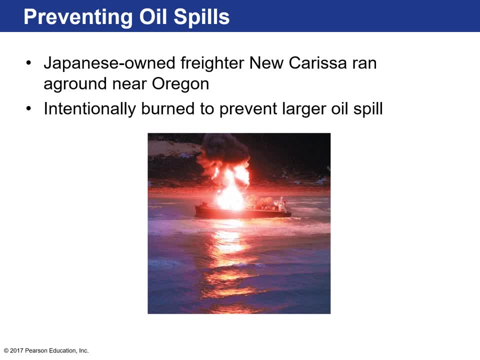 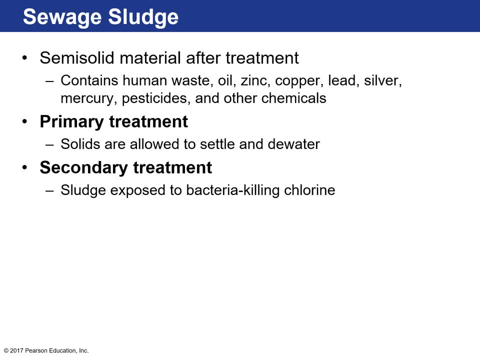 Okay, So it's not a landslide, a larger oil spill. All right, Let's move on to sewage sludge. All right, So that's that semi-solid material after treatment, of course. So all the toilet bowl washing or flushing that we're doing, all that waste water then. 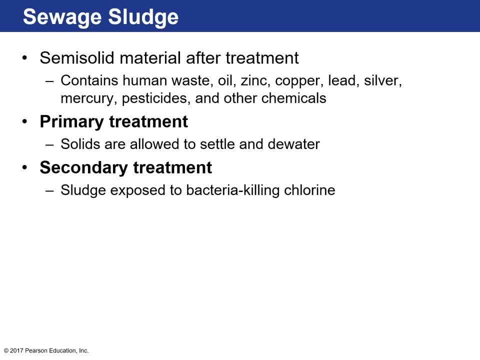 goes to wastewater treatment facilities, human waste oils and copper and lead, silver, mercury, pesticides. All that stuff becomes kind of emulsified, Okay, in this material, solid material. okay, that's the sewage sludge. okay, so the primary treatment: those solids are allowed to settle. secondary treatment: it's exposed to bacteria killing. 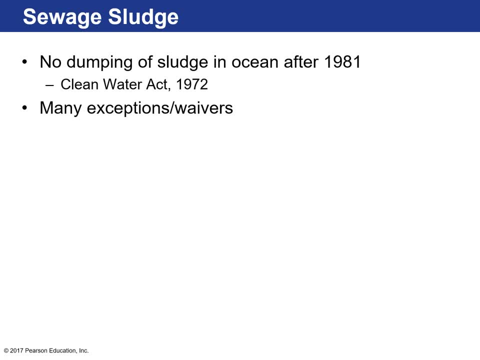 chlorine. okay, so, uh, we used to dump a lot of our sewage sludge just directly into the ocean, just right into harbors, right into coastal waters, um, and that, you know, solved the problem back in that time, uh, but uh, what ended up happening is people like to go to the coast and the beaches to, uh, you, 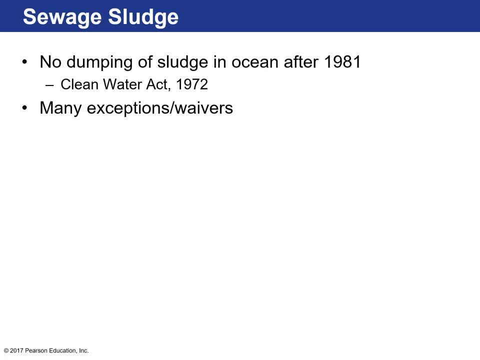 know have do recreational activities and enjoy um the fun. but uh, once the sewage smell started washing ashore, people realized this could be a problem. uh, diseases could be spread that way. um so after 1981, there wasn't you, you weren't allowed to dump uh sludge into the ocean. after that, 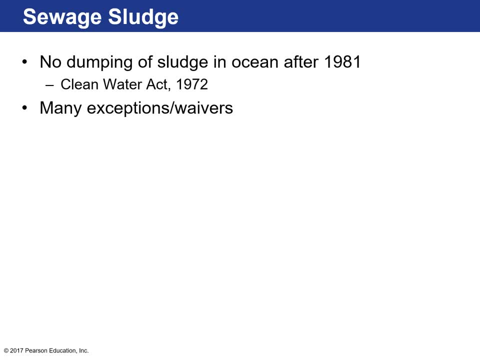 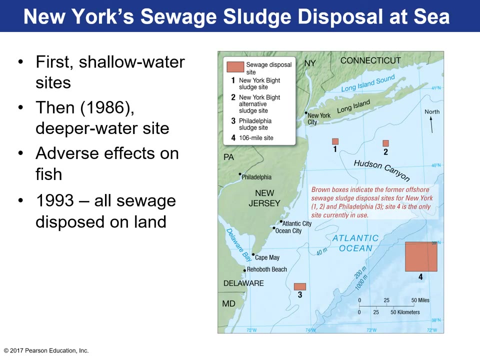 uh, because of the clean water act in 1972. but, uh, they ran into problems. it became really expensive to dump the, the solid waste, onto land, so there were a lot of waivers and exceptions. so into the 80s this continued to happen for a while. okay, uh, in new york. okay, very big city, lots of uh sludge being 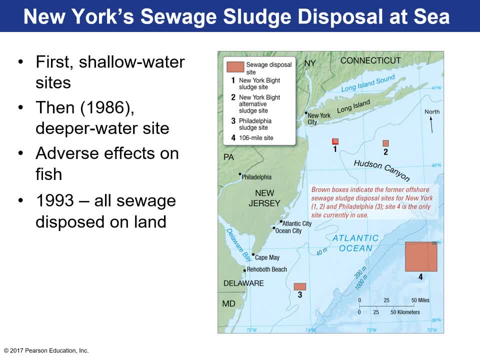 created there. this is where their initial sites were one and two: okay, um, and this was done in um water that was, uh, shallower than 40 meters. okay, that's pretty shallow. so what would happen is a lot of this material would would be pushed towards land because of the incoming tides, um, and that caused 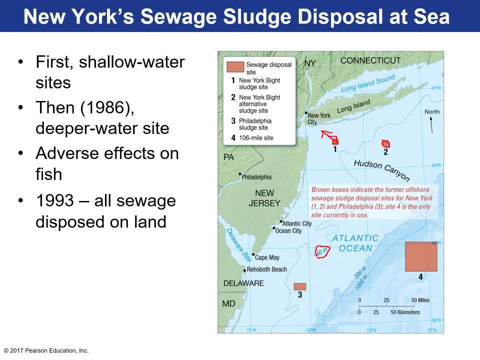 problems. that made the water quality pretty, pretty terrible on the coast of new jersey and new york. okay, um, so in 1986 they decided to change that and have their dumping sites all the way out here. this is the dumping site number four. okay, um, but again this is in deeper water, so beyond about a kilometer of depth, but still, uh, commercial. 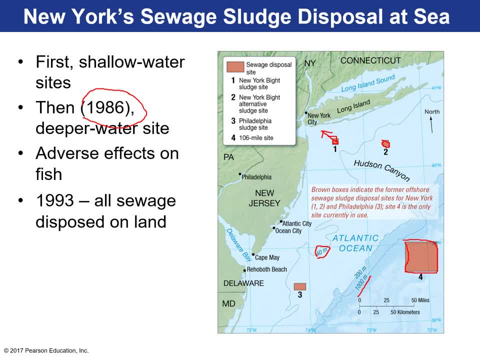 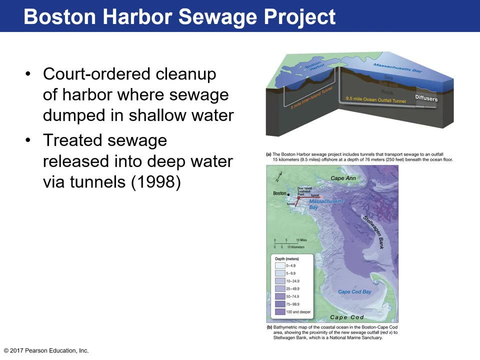 fisheries started complaining that they were uh, uh, catching less, less fish as a result of sewage sludge being dumped out here. so by 1993, uh, it was all stopped and and all the sewage was then disposed on land. okay, um, boston harbor, or boston, had a real big issue with sewage sludge. 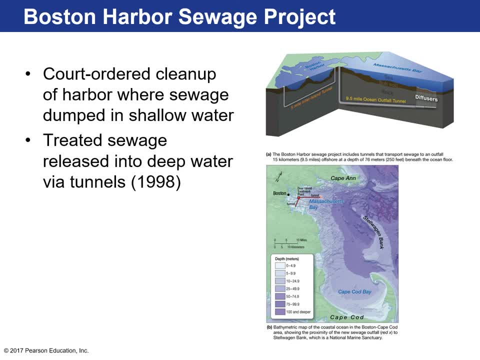 um, they had, they had all the sewage sludge and they had all the sewage sludge and they had all the sewage just go right into the boston harbor and that made it one of the dirtiest harbors in the us- absolutely disgusting, okay. um, and so what they did to alleviate this problem was: 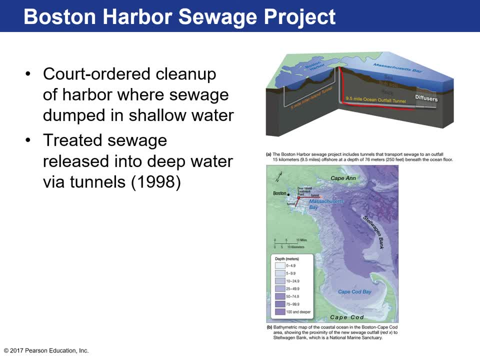 they built a 9.5 mile long uh like pipe with small diffusers to let the sewage kind of slowly trickle out into the ocean, basically into the uh the the sea floor, and then kind of come out into the ocean, and that drastically improved the water quality uh, in the boston harbor area right here. 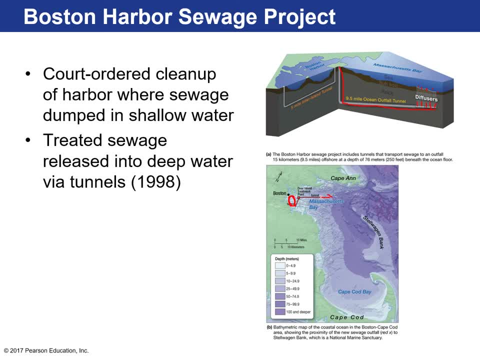 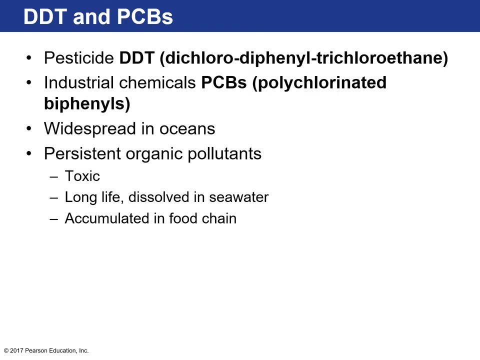 okay, um, so that sewage just slowly let out um into the ocean instead of just being dumped out there, so that improved the conditions in in boston, which is pretty bad. but it cost the- it cost a lot of money to build this uh huge um pipe. okay, all right, let's move on to the next type of pollutant. 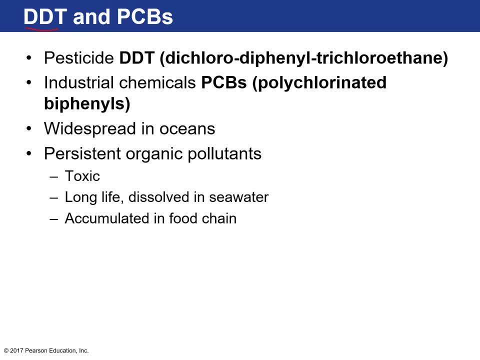 ddt is a pesticide: dichlorodiphenyl, trichloroethylene, ethane- excuse me, that's ddt. and then there's some industrial chemicals: pcbs, polychlorinated biphenyls. okay, they're found everywhere, guys, this is, these are in the oceans. um, we use them without any regard. uh, early on. 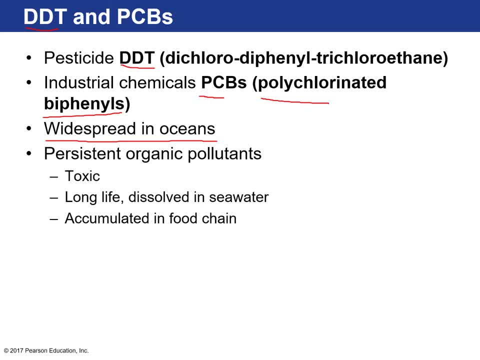 ddt kind of like in the 40s and 50s pcbs during that time as well, but we refer to them as persistent organic pollutants because they're still around today. we can find them in antarctic waters and in soil or ocean sediment near. 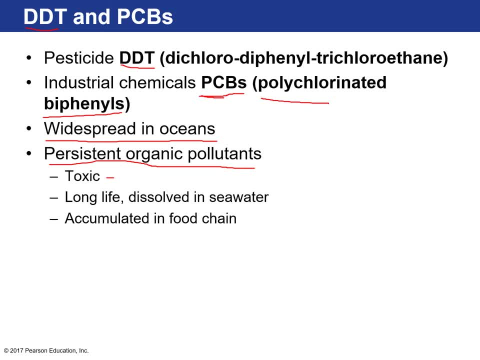 antarctica as well. they're toxic. okay, they are in the oceans for a really long time. ddt has a number of uh, of really adverse effects to organisms- we'll talk about in a second- and the problem is that they accumulate in the food chain, which is a problem- okay, one of the most notable problems, and i'm sure 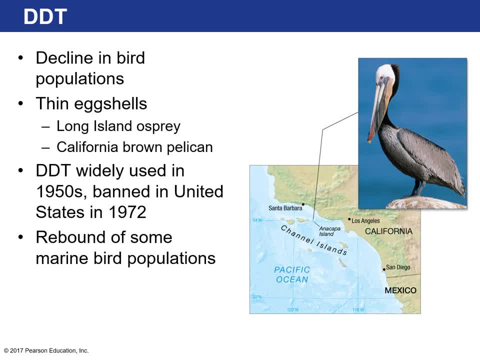 you've heard of this are the way that ddt affects um the bird population's ability to create uh eggs or, essentially, um what happens is if you have ddt uh spilling out into the oceans um pelicans eat the fish and the fish are swimming through the the. 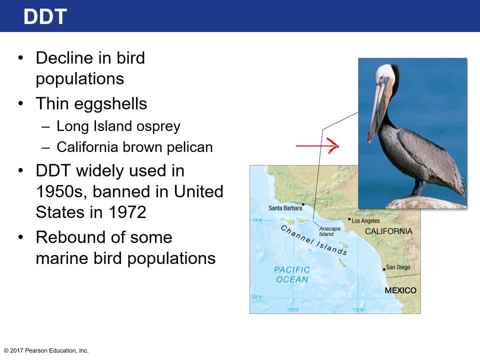 contaminated waters or the or and eating the zooplankton and smaller fish that are around the ddt, so it kind of bioaccumulates and the concentrations increase uh in these marine seabirds and what happens is when they lay their eggs, bloop right their eggshells. 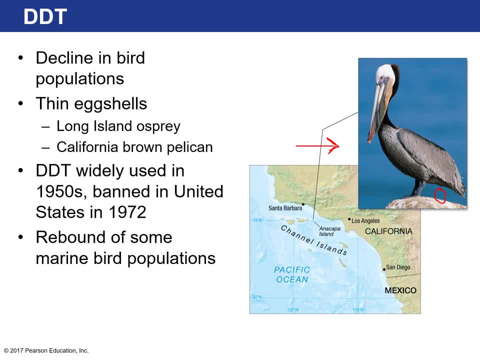 don't have a lot of calcium, because that calcium is being replaced by ddt, and they're too thin so their embryos don't survive. so what ended up happening is that the ddt was replenished with new generations because of these very thin eggshells. 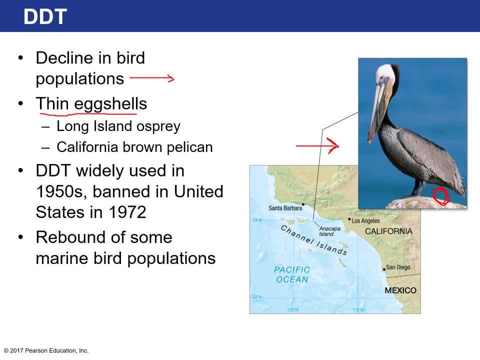 so we saw a huge decline in bird populations and it really threatened the bald eagle. okay, uh. so, along with the california brown pelican, the bald eagle was, um, uh, was stressed because of this and and ddt was a widely used um insecticide, just kind of poured. 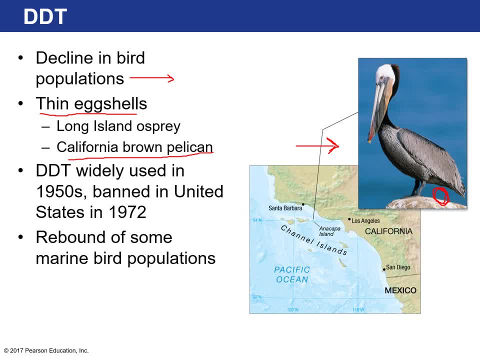 all over crops which, uh which. for farmers, they liked it because it increased their production. but slowly people began to realize, um, that it started killing a lot of organisms and that would have an adverse effect on the environment. okay, um, ddt was banned in 1972 with the uh clean. 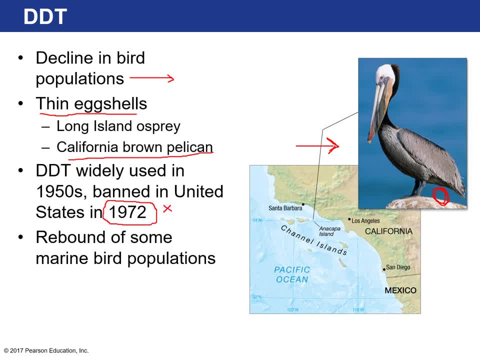 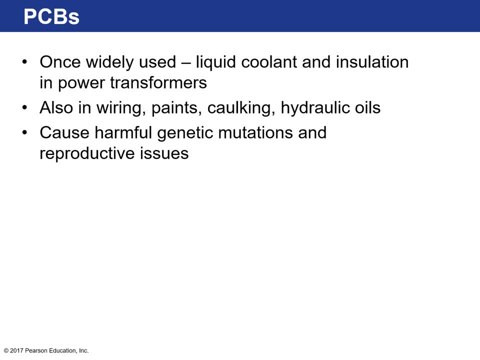 water and clean air act that was passed and that was in large part due to, um, uh, silent spring. okay, that was a book that was published, written by, uh, rachel- oh god, i forgot her name- um, but silent spring is a book that talks about, uh, the use of ddt and how it affected. 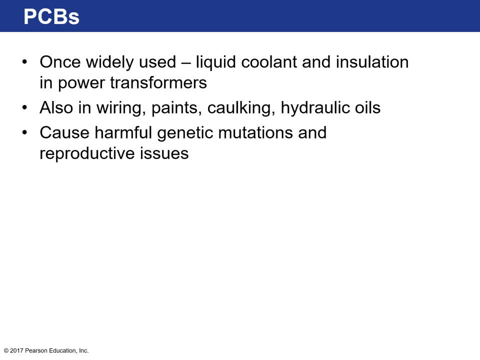 bird populations um, rachel carson, okay, um, and that was really like a paradigm shift and at the beginning of environmentalism and kind of understanding, uh, that these chemicals and and that we're kind of using for industrial purposes or agriculture could have an effect on our our. 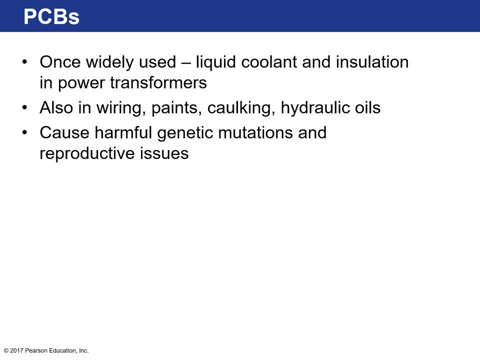 environment, um. so yeah, pcbs- those are um- were used as uh coolants, liquid coolants for refrigerators, um, and there were also uh insulators and also in power transformers. we also use them in paints, caulking uh some hydraulic oils, and they're pretty bad they. 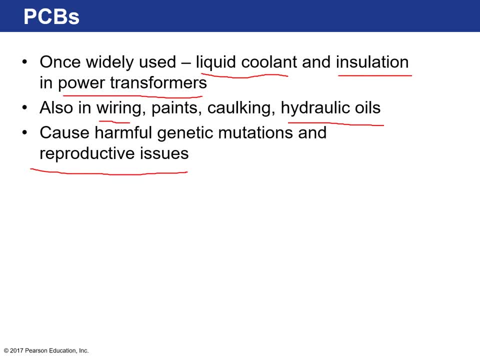 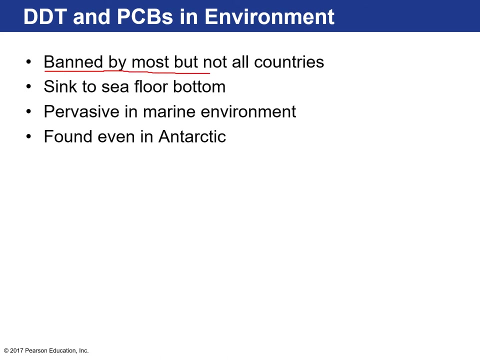 affect our reproductive um uh ability abilities, or just they kind of reduce the reproductive rates. they cause harmful genetic mutations um. so if in, if they're, if you're exposed to them for a long enough period of time and in high enough concentrations, um, you see really adverse effects uh to them. okay. so most of these chemicals, ddt, are banned by most countries. 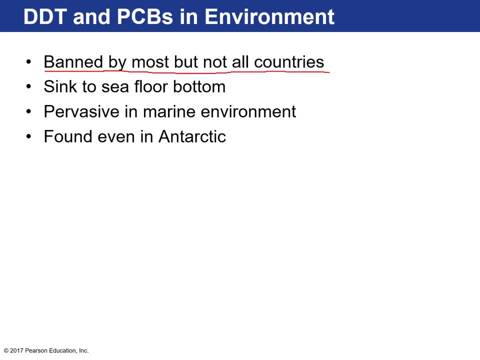 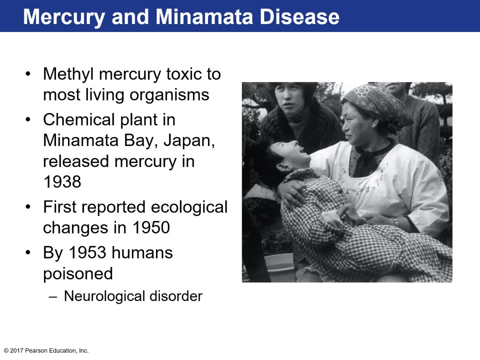 uh, but not all of them, okay. so they sink to the sea floor bottom and we can find them almost everywhere, so they're pervasive. so we even find them in antarctica, all right, so that's, that's pretty bad, but we've banned them here in the us, which is a good thing. okay, all right. the next uh major. 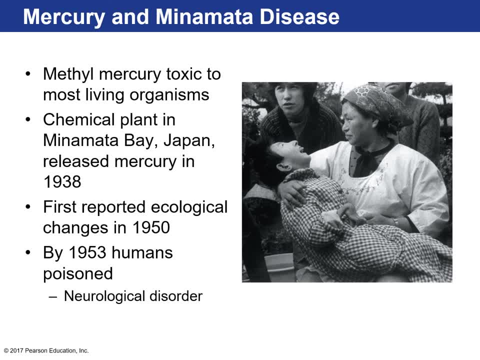 pollutant we'll talk about is mercury. mercury is a, a metal that is found- uh, it's ubiquitous, it's everywhere. it occurs naturally from erosion of certain rocks that have mercury in them, but in large part it's in the environment, because mercury is found in coal, so when we burn coal, oftentimes it's burned into the environment. 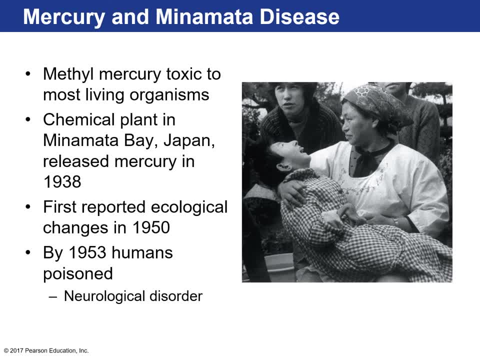 okay and so, uh, so it's basically ubiquitous in the environment, environment and sediment and and in organisms, and you and i, we all have mercury in our bodies. but one, uh, really particularly sad case was, uh, in the 40s, 1940s in um in japan. uh, there was an industrial power plant. uh, not a power plant, but an industrial. 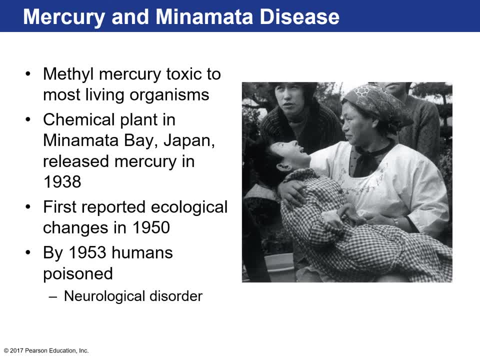 plant that would use mercury to burn down the environment. so they were using mercury as one of the you know the process of creating another chemical and it had a lot of mercury as as a as a waste product, and so they would just dump that into the bay, okay, um, and it was in minamata, minamata bay, okay, so they released. 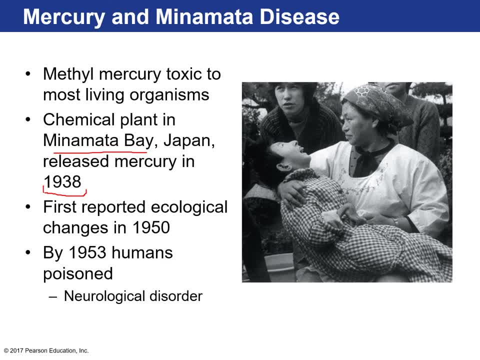 a lot of mercury in the late 30s. okay, um, and what ended up happening is the organisms in that bay started to uh kind of ingest uh allergy and zooplankton and small fish and then they started to eat smaller fish and larger fish started eating those smaller fish and mercury started accumulating. 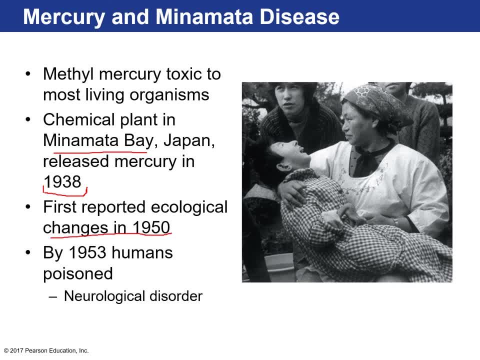 the tissues of these organisms and by the 1950s there started to be really awful effects on the human populations, or the japanese people that lived in minamata bay. um an exposure to mercury in high concentrations caused neurological effects, um involuntary muscle twitching, uh and. 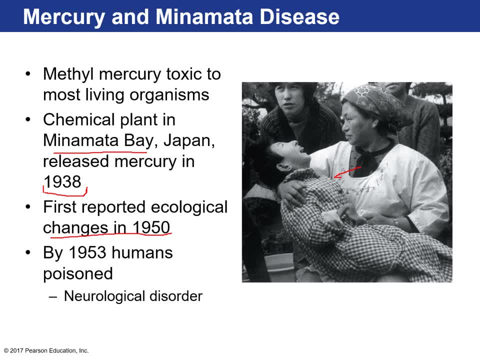 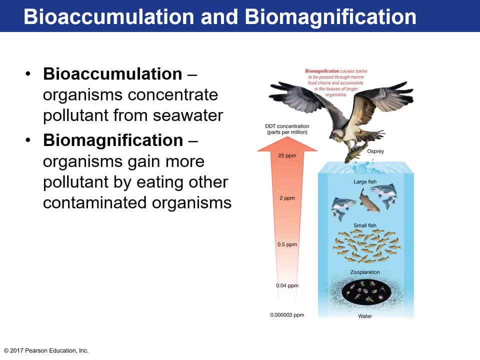 effects, the the development of fetuses and um, children can be born with really problematic mental deficiencies and muscular deficiencies and neurological deficiencies. okay, here you can see a child that was born with a severe minimata disease. okay, so it's really a neurological disorder, okay, and the reason is because the people here in minimana, the japanese people, they ate a lot. 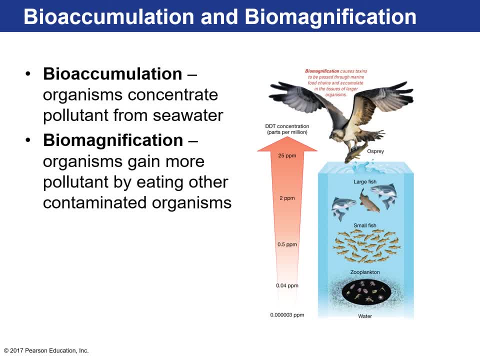 um, in fact the fish markets there, that's the main uh food in their diet, um, and so they would eat fish, you know, multiple times a day, you know three times a day. and what happened was the zooplankton in the water had really small concentrations of mercury from dumping from that uh, from that plant. then 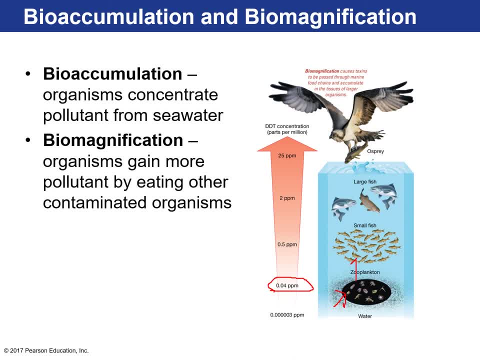 the zooplankton were eaten by the small fish. and as this happened, uh, one small fish will eat many of these small fish, and then the zooplankton. so, as they eat, you know, hundreds or thousands of little, tiny organisms, the concentration of mercury increases and then, as these small fish are eaten, 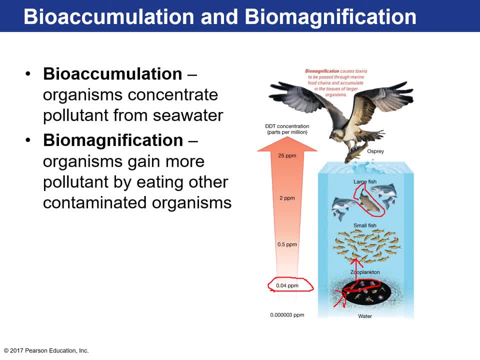 by larger fish like tuna or any other predatory fish. they eat many of these fish that have higher concentrations of mercury, so it accumulates and increases in concentration. so large fish which people would eat, or let's say osprey, would eat these fish multiple times a day. 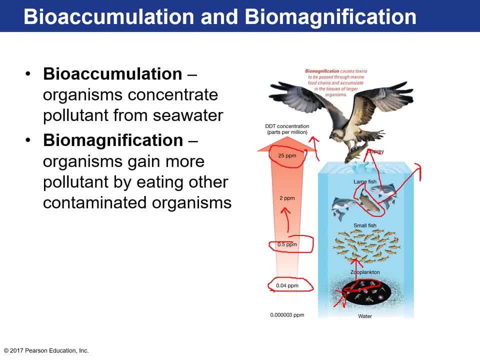 their concentrations of mercury would increase. okay, we call this bioaccumulation, all right, and biomagnification. so the further up you are on the food chain, the higher concentration of mercury are in those uh organisms as a result of eating many organisms that have been exposed to that. 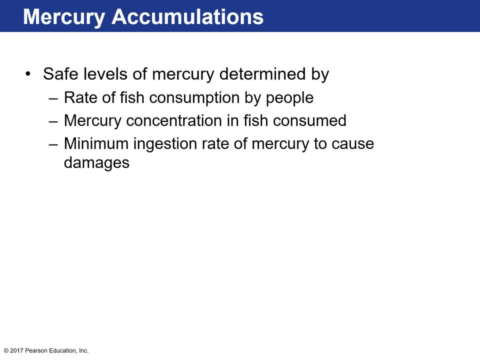 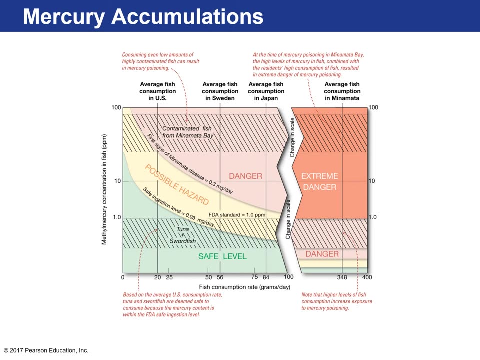 pollutant. okay, so we've determined safe levels of mercury by comparing the, the amount of fish consumption and also the mercury concentration in those fish. okay, and also, what's the minimum amount of mercury we can eat to cause the least amount of damage? okay, here's a chart to check that out. so, um, these are uh organisms that have uh kind of 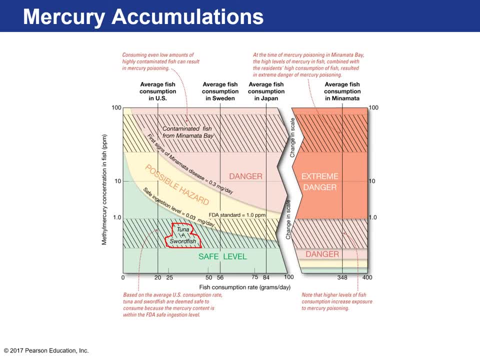 high levels of mercury in them because they're kind of top predators in the ocean so they've bioaccumulated a lot of mercury. so swordfish and tuna. that's why they always give you recommendations when you eat tuna like. let's say, if you're pregnant you can only have tuna like once every two weeks. 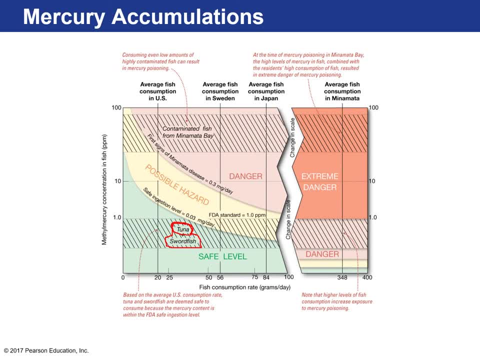 uh, that way, the mercury doesn't affect the um baby that's developing in your body, but here it is. so, uh, the average us citizen consumes about 20 grams of fish a day. okay, and if that's, uh, this is considered a safe level at this area. okay, um, 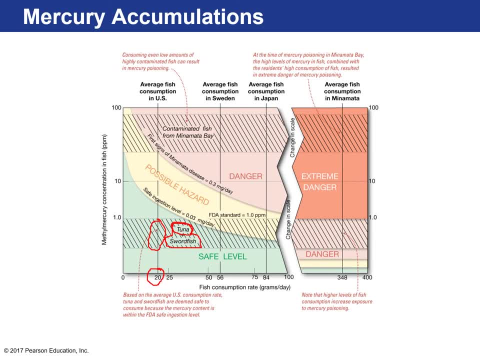 if you go to- uh, this is average us consumption people in sweden. they have a high fish diet, so, uh, if you're eating fish that's not being contaminated by a plant, that's just natural mercury that's in the oceans. that's around this level. so so swedish people are kind of safe eating. 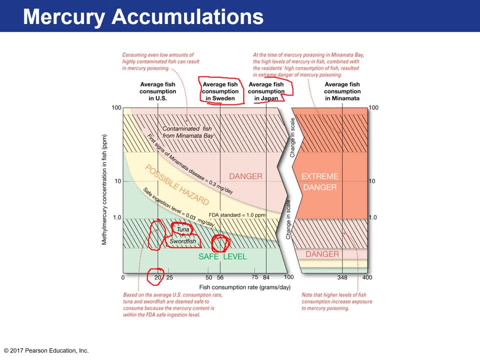 at that level. and then in japan they eat a lot of fish three times a day, um, or about 84 grams a day. maybe not three times a day, twice a day or so, but a lot of fish in their diet and still that's very safe if you're eating, uh, from waters that aren't contaminated with mercury and even 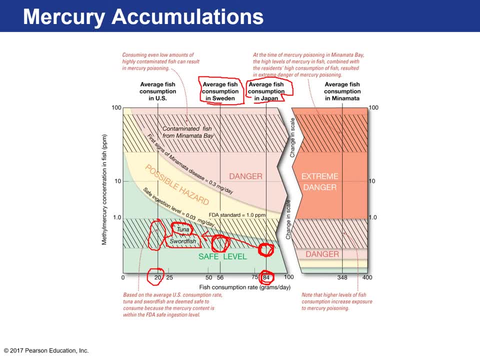 you know top predator fish like tuna and swordfish. however, this over here is the methyl mercury concentrations in the fish itself and in the 1950s in japan and minimata bay, this was the concentration of uh mercury in the fish. so even if you were an american, only eating 20 grams of 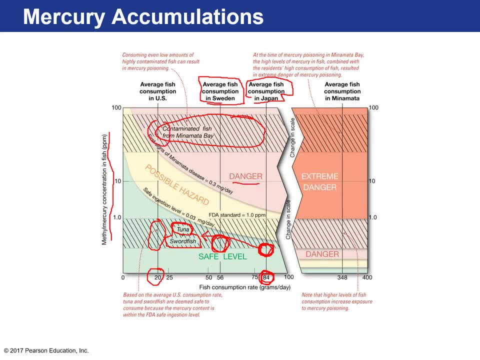 fish per day, this would be dangerous okay, and if you were eating 10 grams of fish per day, this would be dangerous okay. so this is the average fish consumption in minimata. so most people there were eating over 348 grams of seafood a day. they were in this. 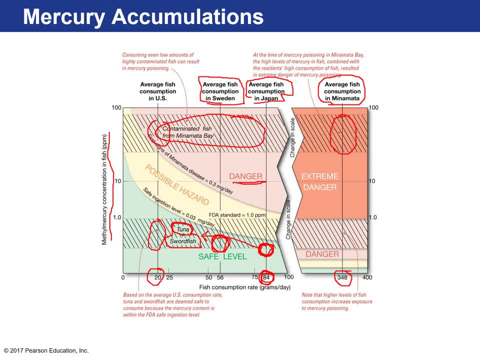 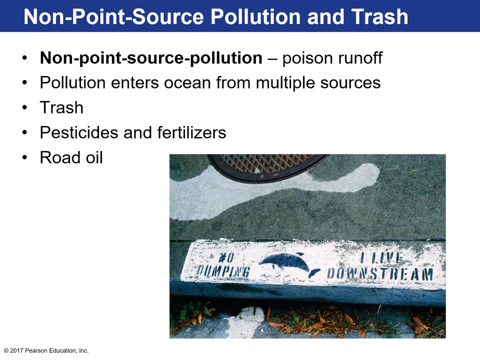 extreme dangerous territory which caused that disease and a lot of people died as a result of this. okay, and just to give it some perspective, uh, one can of tuna, like your can of tuna, is about 100, 100 grams of fish. uh, 100 grams of, yeah, tuna, right here. okay, let's move on to non-point source. 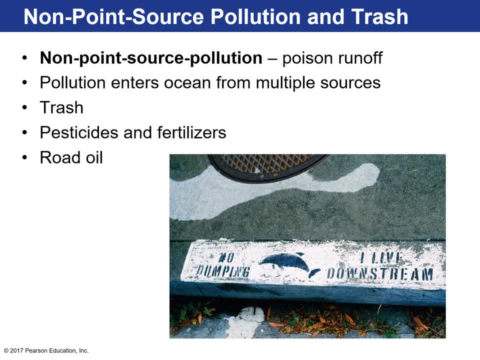 pollution. okay, so this is a lot of different types of non-point source pollution. okay, so there's plastic, pesticides, fertilizers, road oil, trash- it's just anything where there's runoff from land and it can come from multiple sources. so there's a lot of different types of non-point. 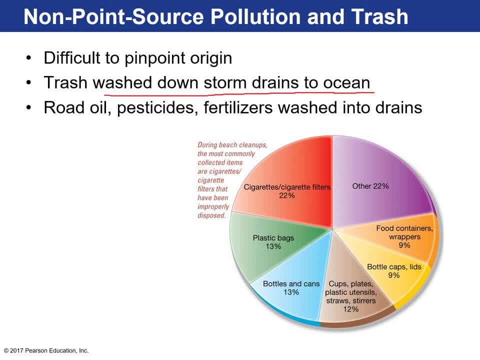 source pollution. okay, it's hard to pinpoint its origin. it's just trash that's washed down storm drains into the ocean. that's why you got to be careful with what you use. sorry smokers, you guys are contributing a lot to the oceans. i know smoking is not very popular amongst the younger. 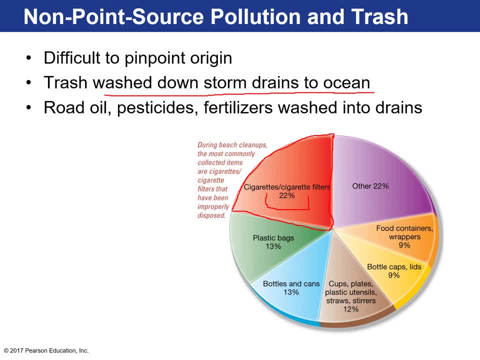 generation, but a lot of cigarette filters end up in the ocean. almost like a quarter of non-point source pollution are cigarettes. food containers and wrappers, bottle caps and lids, plastic utensils and straws. bottles and cans and plastic bags are a big portion of this. others just break down of all. 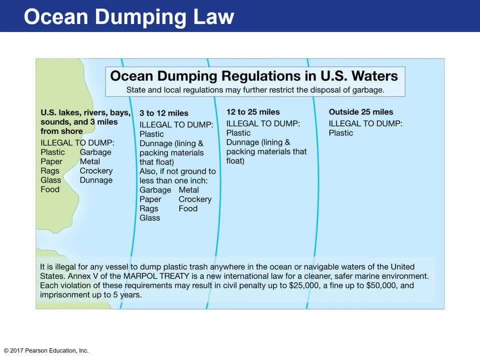 kinds of other different plastic materials. excuse me, here are the ocean dumping regulations in us us water. so, um, if you're within three miles of the coast, you can't dump any of these materials. all right, it's illegal to dump any of that stuff. um, then, when you go out to three to twelve, uh it. 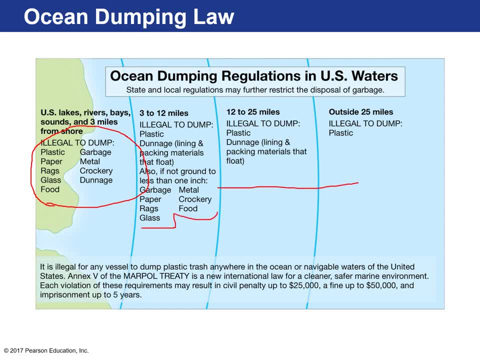 kind of lowers down a little bit and once you get outside 25 miles, uh, the only thing that's illegal to dump is plastic, okay. um. so yeah, when cruise ships kind of make it out into the ocean, uh they can- just you know that's a terrible cruise ship- they can kind of dump out their sewage, right. 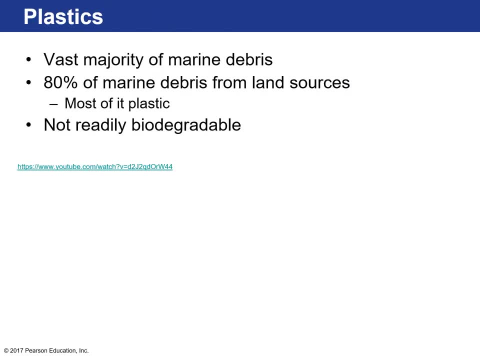 into the ocean, yay, cruises, okay. so the vast majority of marine debris and nine-point source pollution in the ocean comes from land sources and most of it's plastic, and plastic is not biodegradable, not readily biodegradable. what that means is it's forever. so every time like you grab 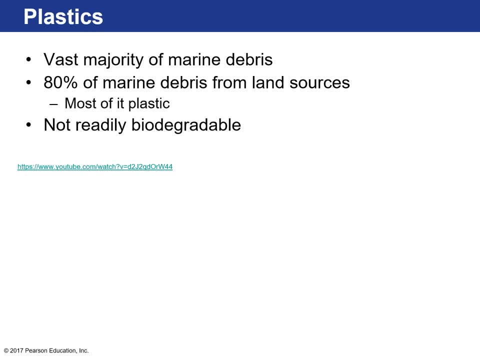 a piece of plastic to grab a donut and you eat that donut and it's done and you throw away that piece of plastic. that's forever. that's going to be there forever. every time you use one of those- you know, a toothbrush- and you 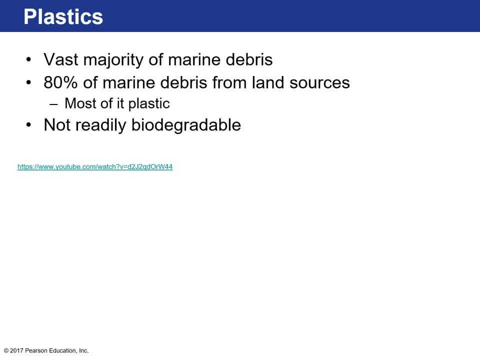 throw away that toothbrush that's made of plastic. that's forever. um. anytime you floss your teeth using one of those plastic flossing tips, that's forever, um. so really, we have to keep in mind all the things that we use, uh like single use plastics. those last forever in the oceans. they. 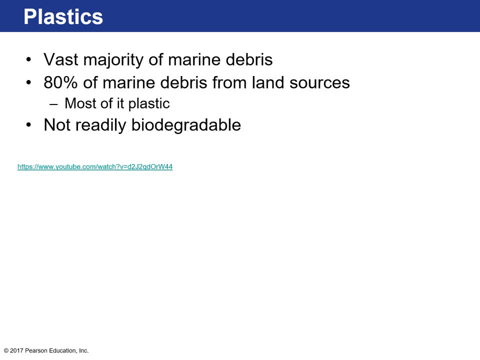 don't really biodegrade. um, there's a youtube video here- i won't, we can't watch it- and this is a video of a sea turtle with a straw stuck up its nose. you can play the sarah mclaughlin music on the background and shed. it's here, but it's pretty bad, okay. so yeah, plastics entangle in fish and 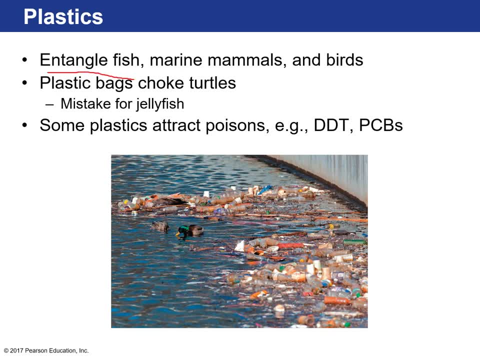 marine mammals and birds. okay, um, you've seen that. you know like they can choke from it. uh, plastic bags in particular kind of float around the ocean and they can kind of sink a little bit and a lot of times sea turtles will mistake it for jellyfish or sea turtles will mistake it for. 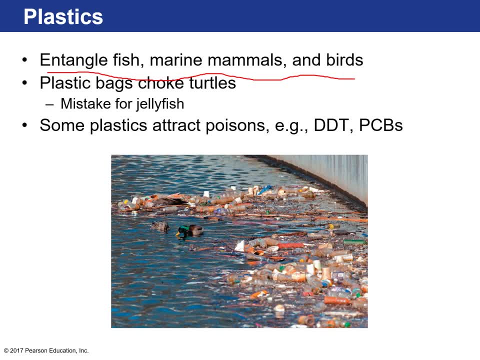 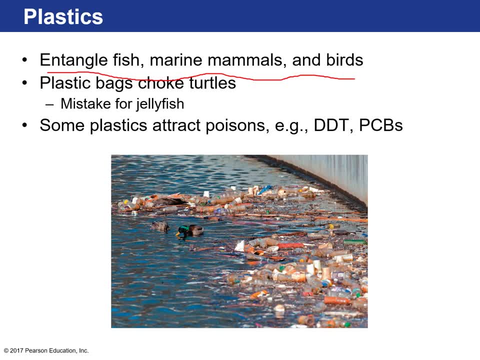 publix, walmart, man, they're bagging one item per bag. the best thing to do is is: uh, really, bring your own bags. or, if you have to use those single kind of use plastic bags, you can bring them back to publix to recycle them. okay, in addition to that, a lot of these plastics have 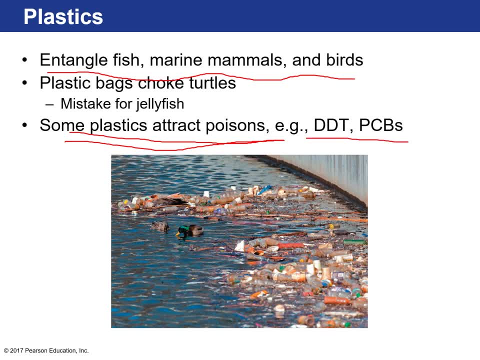 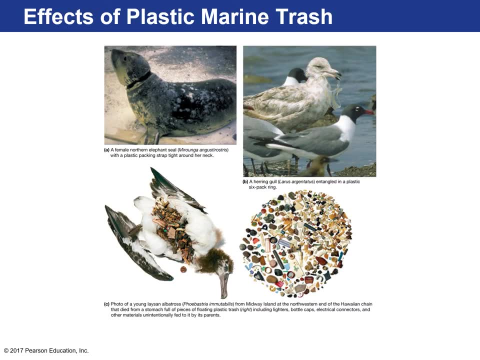 harmful chemicals in them, them ddt and pcbs, pahs, for example. okay, that poor mallard has to kind of wade through all that trash, okay. so here's some examples. here's a sea lion, you know, entangled by a piece of plastic. it affects 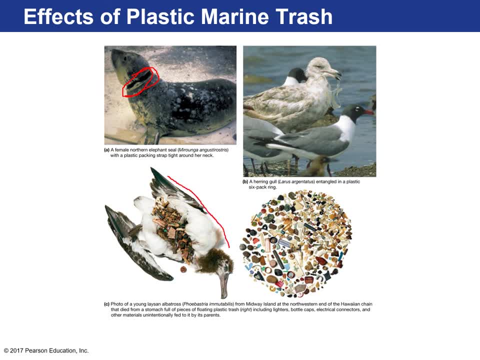 its growth. okay, here's a dead seagull, um, and after it's died they kind of go through its guts and they find all different types of pieces of plastic. look, you can see lighters. you can see little flossers. you can see, uh, just a bottle cap toothbrush handles. that's pretty bad. straws, okay, plastics. 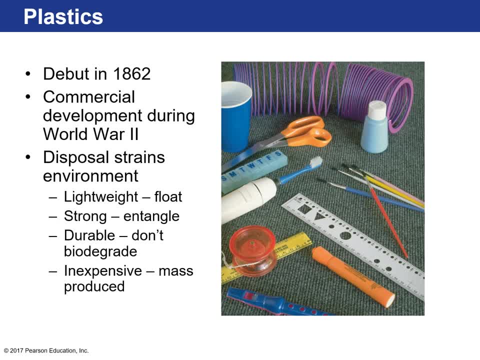 kind of made their debut in 1862. um, they were developed by the uh uh, by the army early on because it was a very, um kind of important materials: very cheap, lightweight, very strong and durable, um, and inexpensive to produce. so plastics were kind of like a great new material. 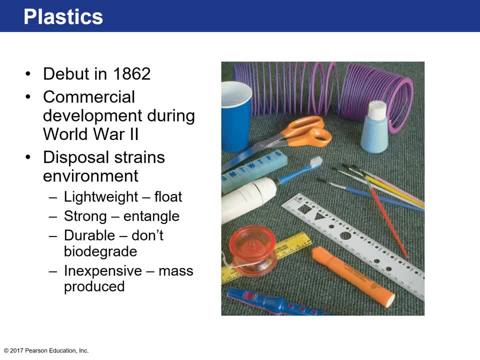 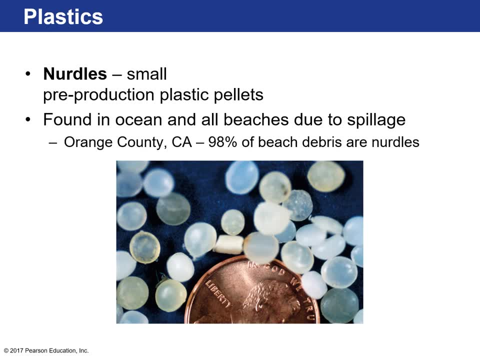 okay, and and what made them so great also kind of makes them bad for the environment. okay, in the production of plastic um, you have these byproducts called nurdles, these really small little circular pieces. a lot of times they use it for packing in material um, but they're for use for pre-production of plastic pellets. they're found in every ocean. okay. 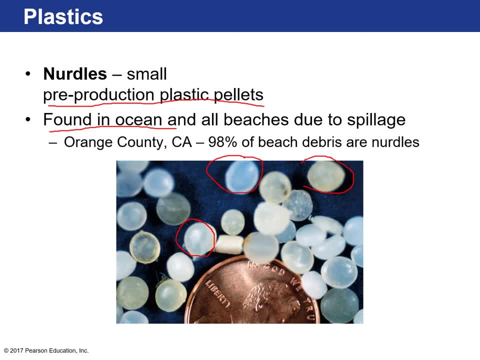 they can be confused for sediment because they're kind of clear. they look like little pieces of um quartz grains or something. but nope, that's plastic. that's what you're digging your feet in- a lot of uh, in a lot of uh. the beaches in florida and in california- orange county, california, for. 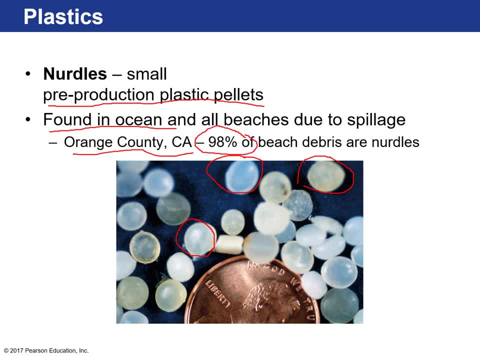 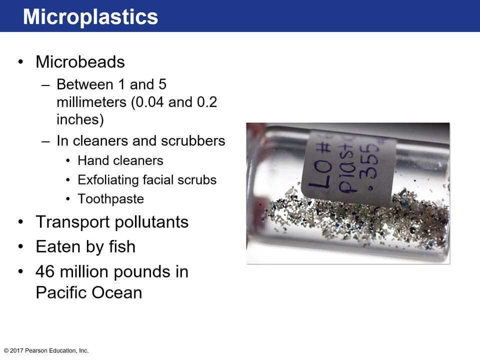 example, southern california, 90: 98 of the debris that's in the sand are actual nurdles that are in the water. they and what happens is they spill off container ships and they float around in the water for a while and that's the thing. like plastic flow, okay. um, what's coming out? uh, in research nowadays, 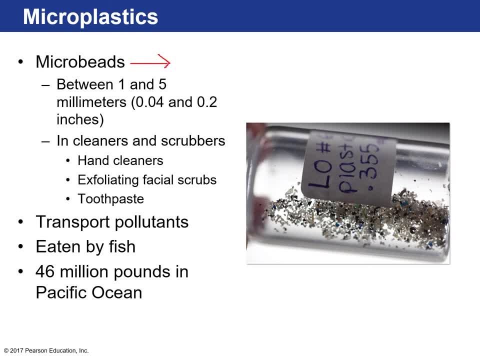 are microplastics- we're starting to kind of figure out what's going on here- and micro microplastics are essentially any plastics that's uh smaller than 0.04 uh to 0.2 inches, okay, between one and five mil meters um, and this is material like, like can come off your clothing. 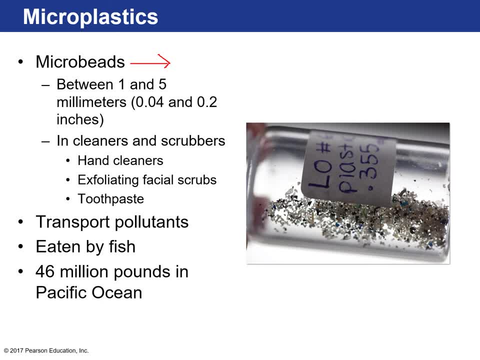 like microfiber. plastic is uh. a lot of times you cannot actually use those um plastic fibers. okay, if you have a shirt that's uh or a jacket that's waterproof- a lot of times they use plastic microfibers in them- or a shirt that's made of polyester, and every time you put that load 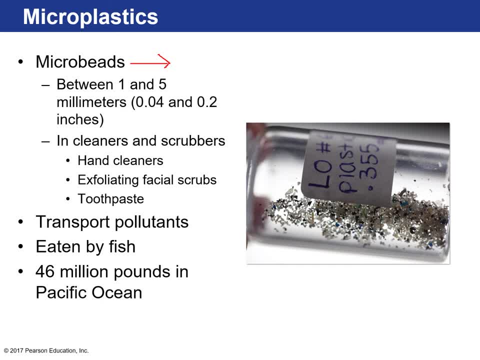 into the, into the washer. those microfibers come off your clothes and they go right into the wastewater and that eventually goes into the ocean. um, you also find these microbeads and hand. those things were like exfoliation microbeads. don't buy those things, because as soon as you 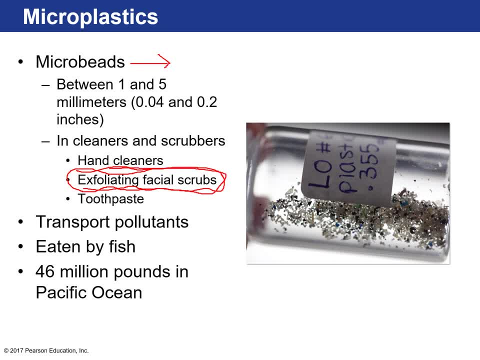 wash your face with them. those plastic beads just go right into the drain and out into the oceans. okay, sometimes you even see them in toothpaste. i wouldn't recommend buying those either, but this is, uh, dangerous. look, here's a vial filled with a lot of these little microbeads. the reason why it's 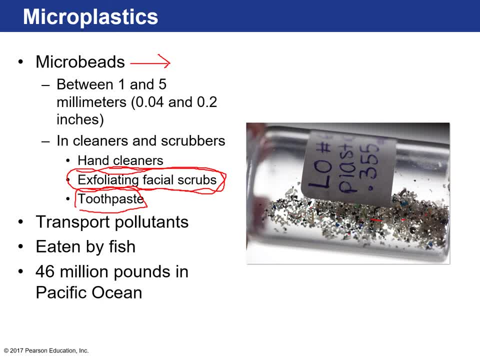 dangerous is because marine organisms will ingest them and they help transport a lot of those pollutants that we talked about earlier, like pahs and stuff like that. they're eaten by fish and guess what happens when you eat fish? then they go into your bodies. no right, so about 46 million. 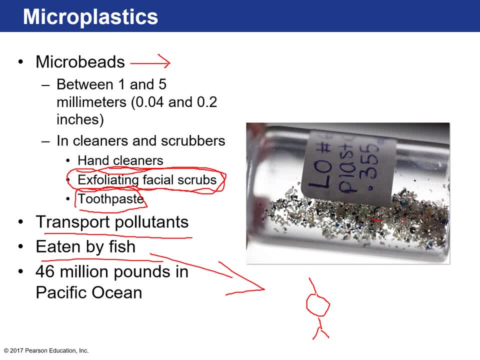 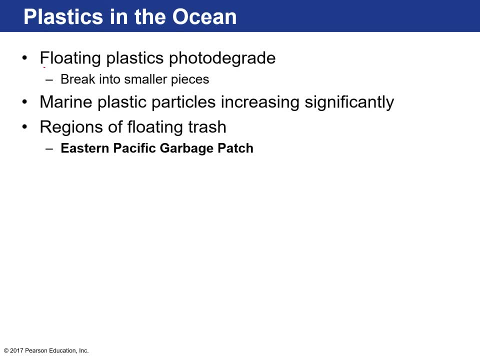 pounds of this is released into the pacific ocean, okay, which is pretty crazy, all right. um, and floating plastic on the ocean surface, um gets hit by the sun and the sun kind of breaks it down into smaller and smaller pieces and those smaller pieces can be ingested by fish. 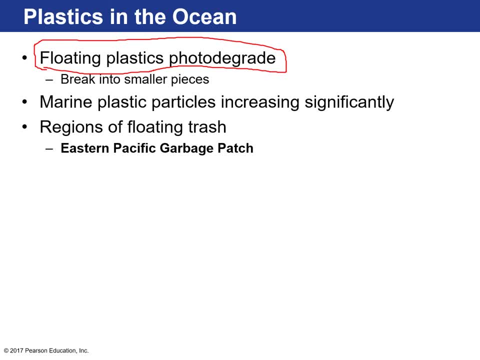 which, when, which, then we ingest. so and in a small kind of long about way, we're kind of poisoning ourselves with this plastic. so marine plastic particles are becoming a significant source in the oceans and it's getting really dangerous, okay, and there are entire regions of the ocean of floating trash- uh, the eastern garbage. 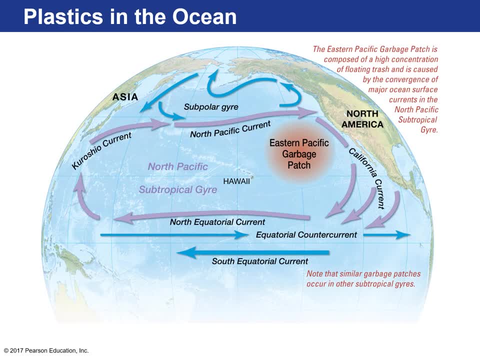 pacific garbage patch which forms over here. remember, this is the uh clockwise, uh currents that form the north pacific gyre. okay, that that picks up trash from all over the pacific and it accumulates in this entire area. some estimates, uh, say that it's about the size of texas. okay, so i don't know what texas looks like, uh, texas. 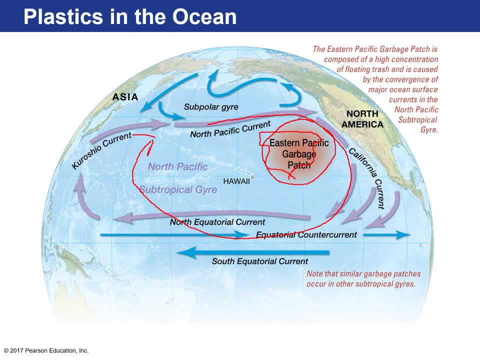 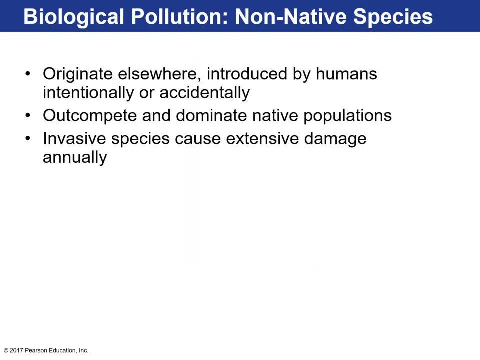 okay, this is huge. it's a giant floating garbage patch, uh, which is, you know, shameful really, um and uh, yeah, so plastic is. my recommendation is: try to use it as least as as little as possible. we have power in the fact that we can choose to purchase what we want to purchase. 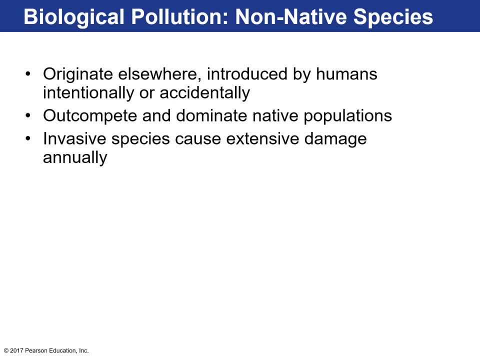 and then so try to find products that have the least amount of plastic as possible. okay, and you can see that a number of companies are kind of moving towards less and less plastic, which is a good thing. all right, all right. the last type of pollution is what we refer to as biological. 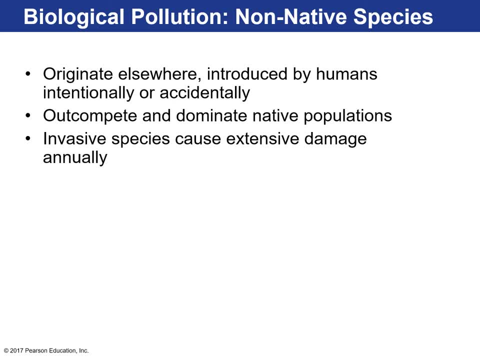 pollution, um, and essentially it's just invasive species, okay, um, and there's organisms that originate elsewhere, and then there's education organization that continues to have that power as well- introduced to new environments by humans. okay, and so what happens is they out-compete and 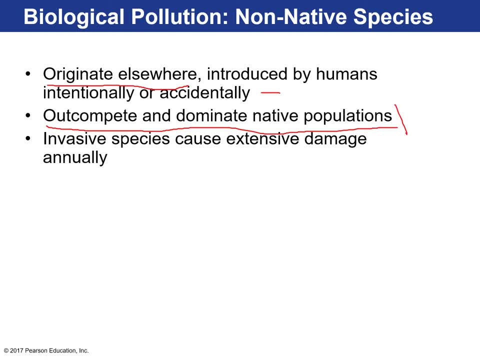 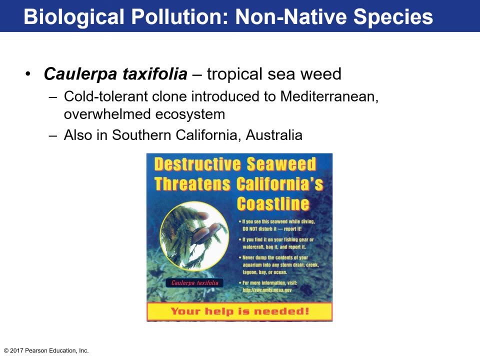 dominate the native populations. You might be familiar with this in the Everglades, with Burmese pythons taking over. okay, so they can cause extensive damage into ecosystems In the marine environments in California. the authors are from there, so there's this tropical seaweed. 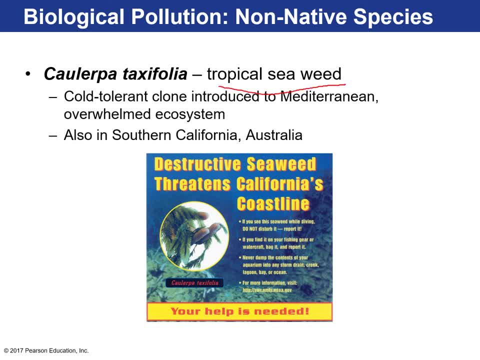 that's really kind of taking over the kelp forests in this area and in California they have kelp forests, which are these kind of large algae that grow, and then they have sea otters that live in them, sea urchins and stuff like that. a very complex ecosystem and this tropical 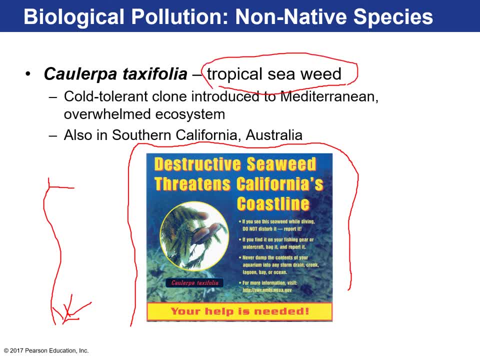 seaweed is kind of taking over that area and really affecting that ecosystem and the reason is because people want to have saltwater aquariums With this easy-growing tropical seaweed and then when they realize it's too expensive or they don't want to keep this tropical nice aquarium, they just dump it into the toilet or into a storm drain. 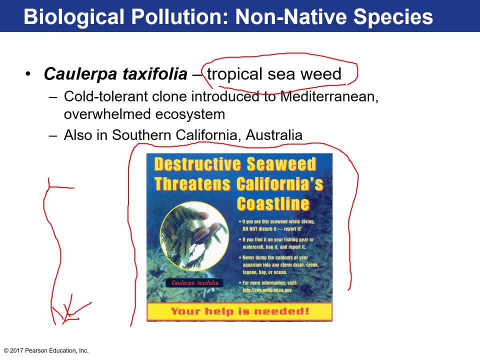 and then that invasive species goes into the California waters and that's pretty bad. Here in Florida, what we've been dealing with is lionfish. That's an invasive species that's all over our coral reefs, which is pretty bad. In fact, you can get paid for hunting them. 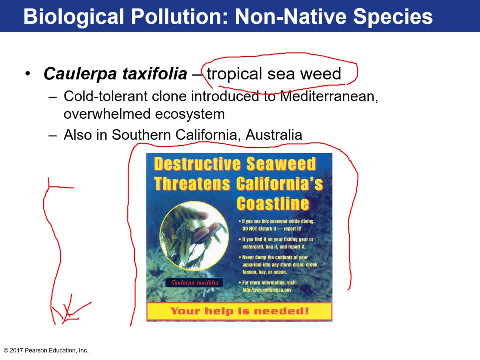 so if you go out snorkeling, you can take a little speargun and you can get paid for hunting them. so if you go out snorkeling, you can take a little spear gun and shoot a lionfish, because they're really detrimental to the coral reefs in Florida. 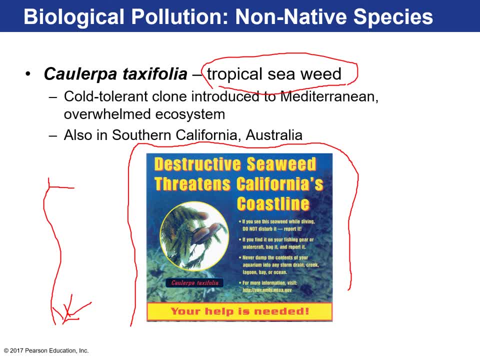 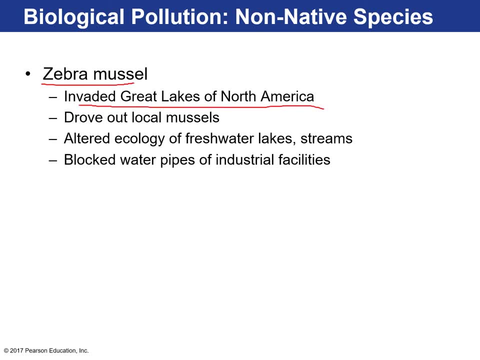 because they're out-competing a lot of the native species there. Okay, another example is a zebra mussel. This is in the Great Lakes. It invaded because it kind of latched onto boats that went into the Great Lakes. It drove out the local mussels, altered the.